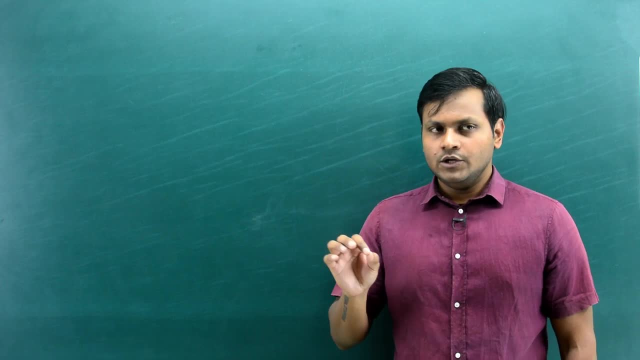 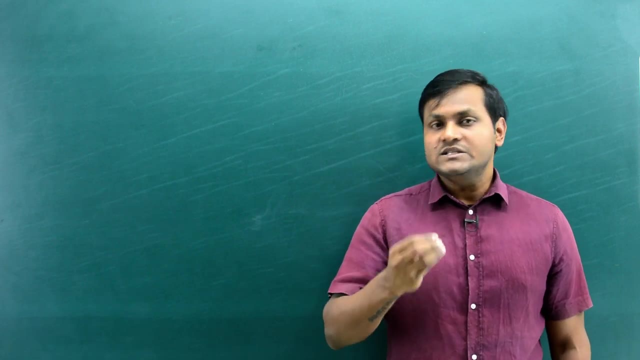 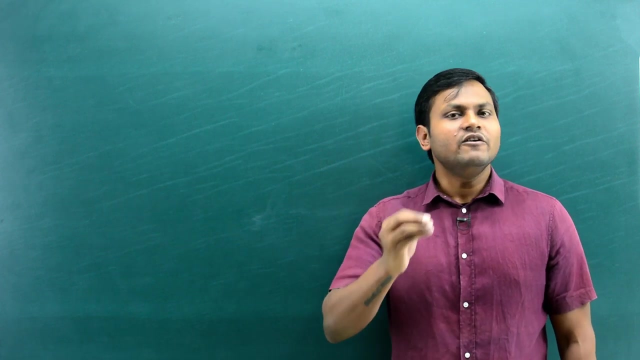 it becomes very necessary to classify them, to organize them into groups or families, so that we can have a better understanding of what these particles are, of what the elementary particles, the constituents of matter, are. One such family of particles is known as the lepton family. 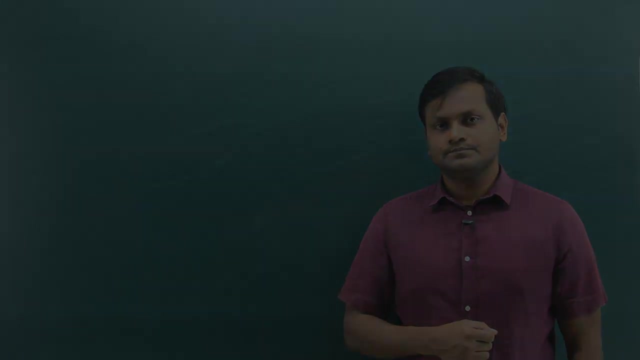 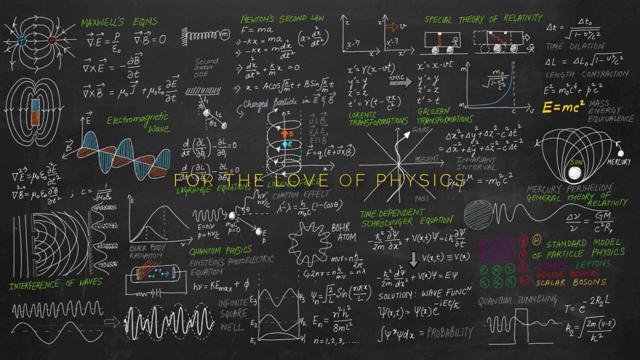 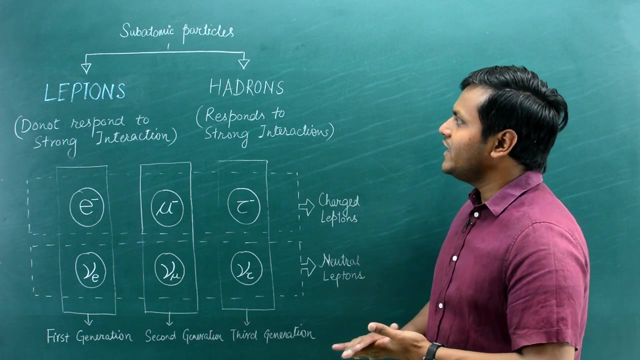 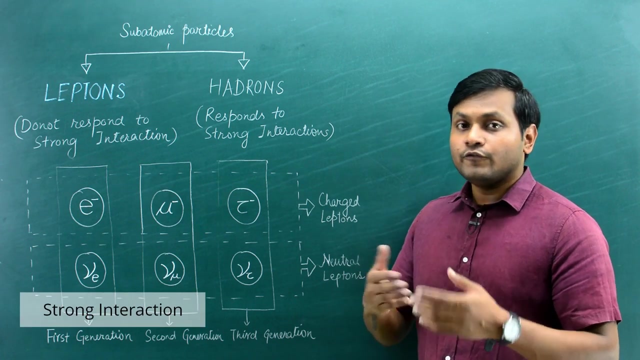 which is what this video is all about. Okay, so all these subatomic particles, we can classify them based on whether or not they participate in the strong interaction. So there are four forces out there. right, You have gravity, you have electromagnetic force. 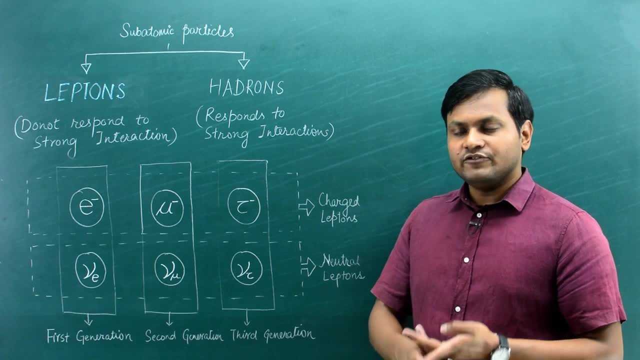 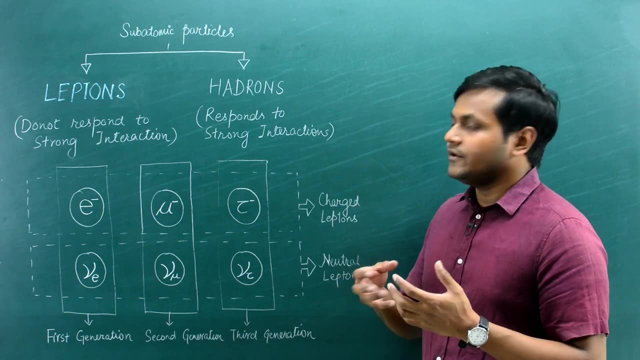 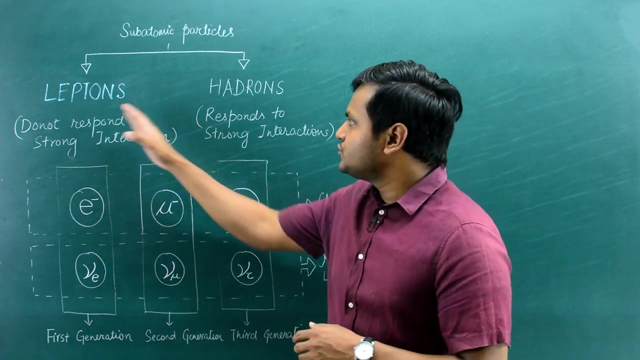 you have strong force or the weak force. I have talked about these forces in one of my previous videos. Now, based on whether or not these subatomic particles respond to the strong force or participate in the strong interaction, we can say that there are two groups of particles. 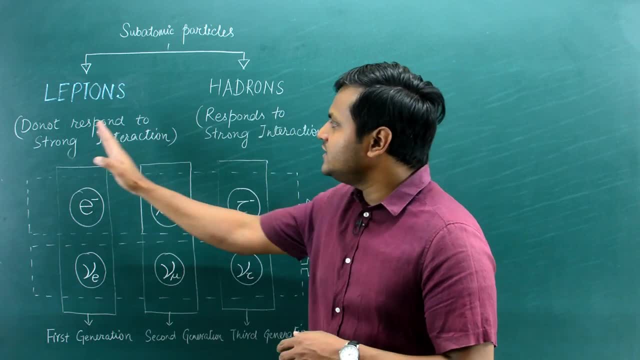 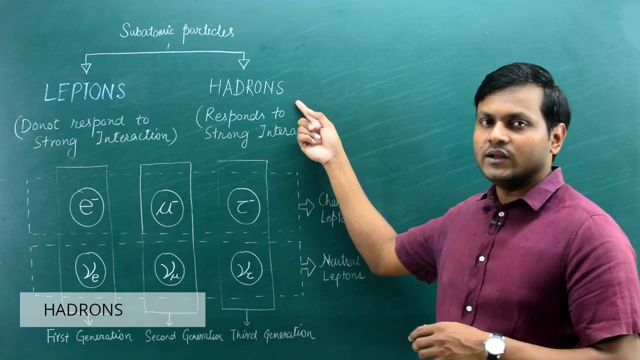 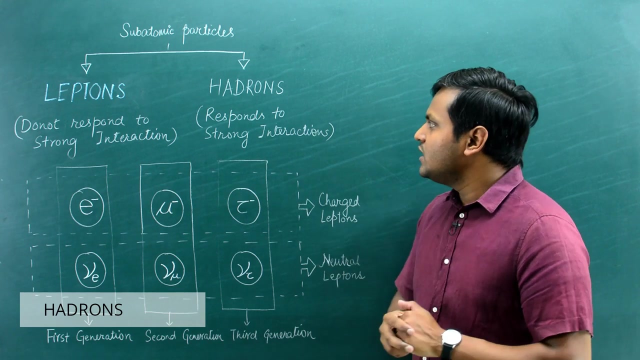 One that do participate in the strong interaction, The other that do not. So the group of particles that do participate in the strong interaction are known as hadron particles. So these are particles like Neutrons, Protons and particles which are further made up of Quarks. 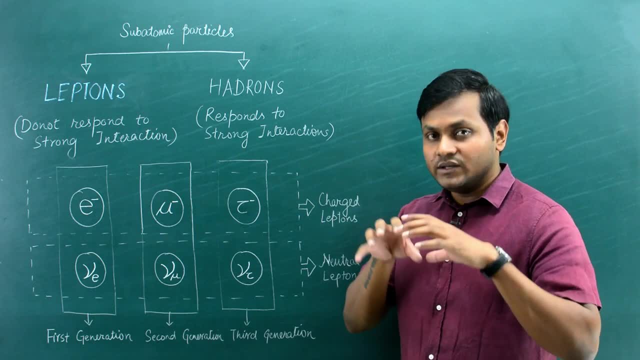 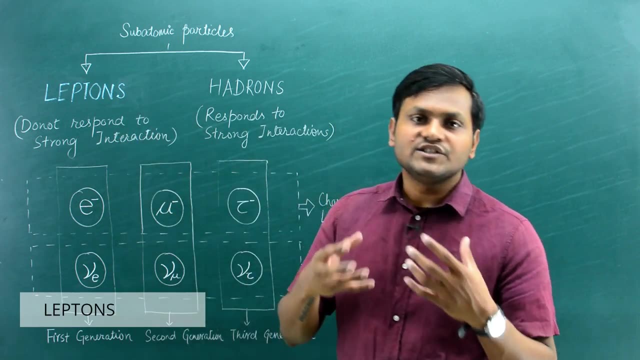 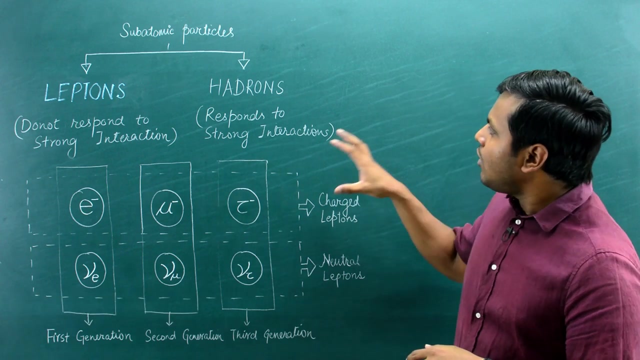 These are particles that respond to the strong interaction. they participate in the strong force. On the other hand, you have the lepton family, which are particles that do not respond to the strong interaction. they do not participate in any kind of a strong interaction. so I'm going to talk. 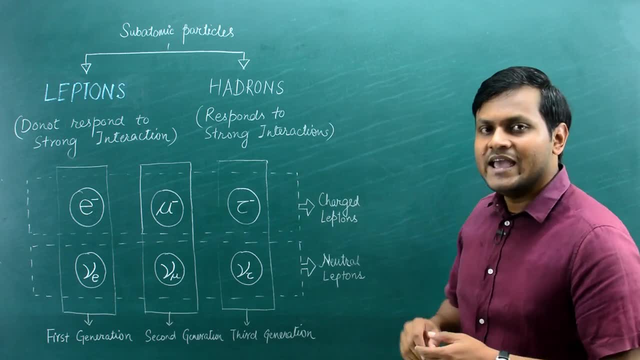 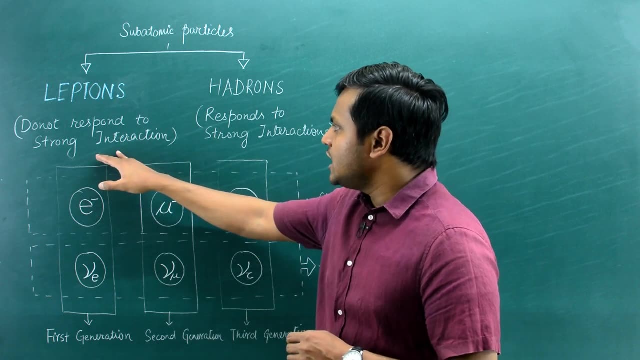 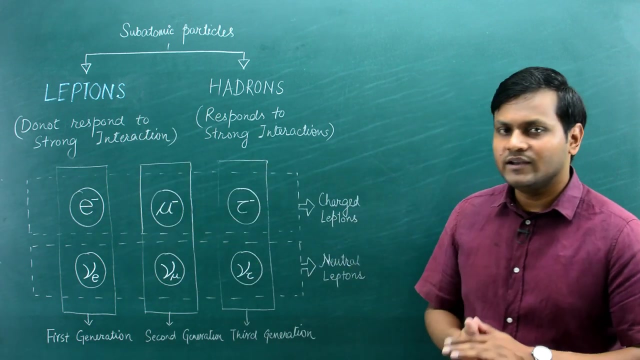 about hadrons and the particles constituting hadrons in a separate video in detail. in this video, I want to talk about this lepton family of particles, these particles which do not respond to the strong interaction, and, as it turns out, these lepton family of particles essentially consists of six. 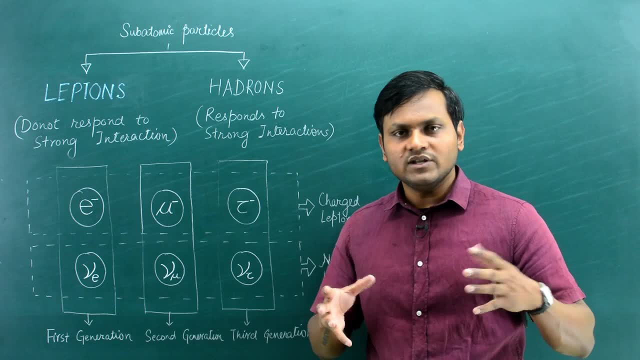 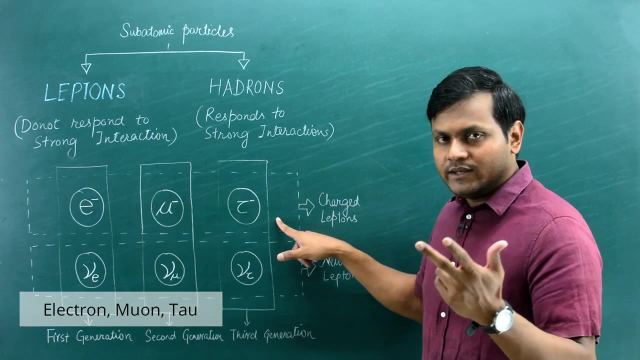 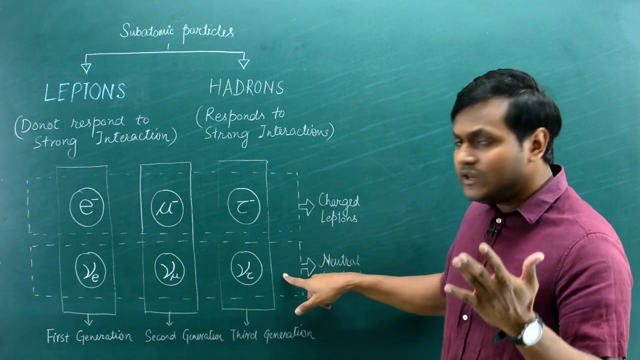 particles. you have the electron. you have heard of the electron is a very common particle. it's part of the atomic structure. you have the electron. you have the muon particle, tau particle and their associated neutrinos. you have the electron neutrino. you have the mu neutrino, the taonic neutrino. so 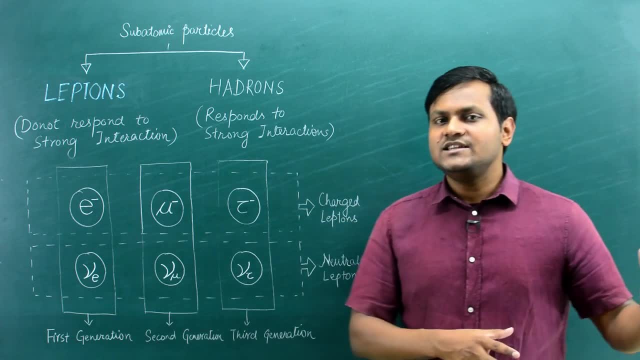 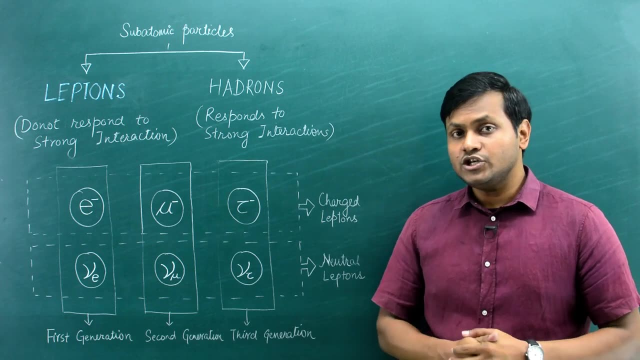 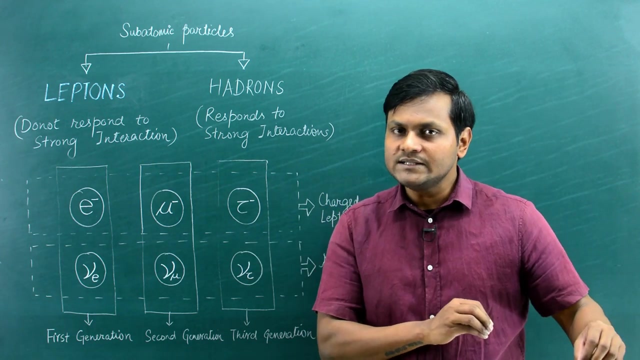 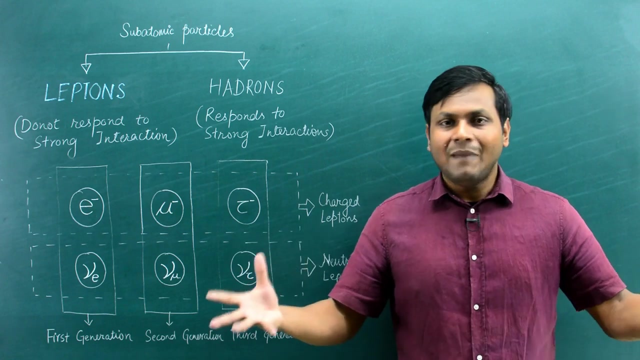 essentially you have six particles and their antiparticles, which constitute what is known as the lepton family. these are essentially elementary particles in the sense that they are not made up of further smaller particles, but they are rather few of the fundamental building blocks of our matter in this universe. they cannot be broken down into. 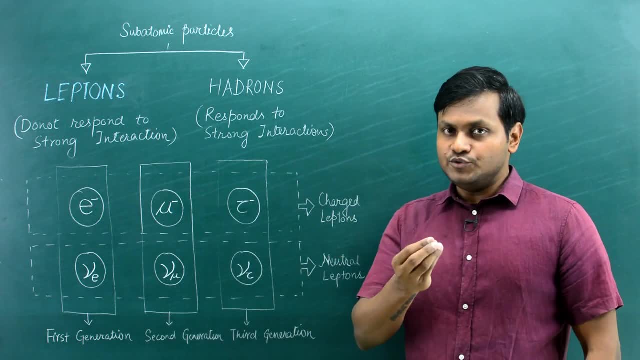 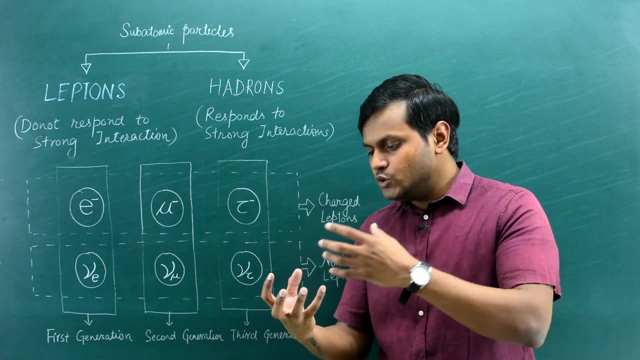 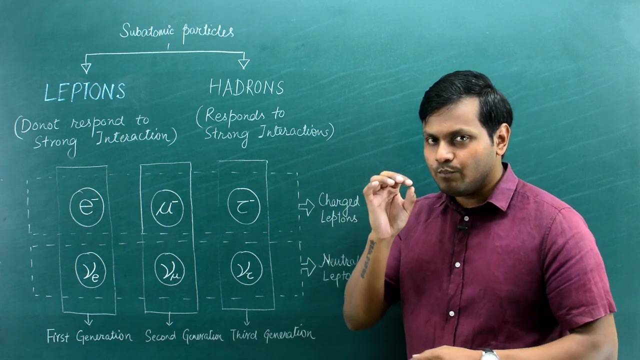 smaller particles. they are point mass objects in the sense that they do not occupy any kind of a space, like, for example, if you have a ball. it occupies some space, it has a size, it has a shape, it occupies a particular volume, but these particles, they do not occupy any space, they are point mass, elementary particles and we can 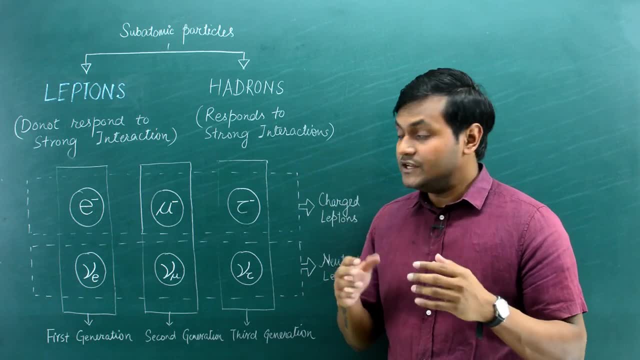 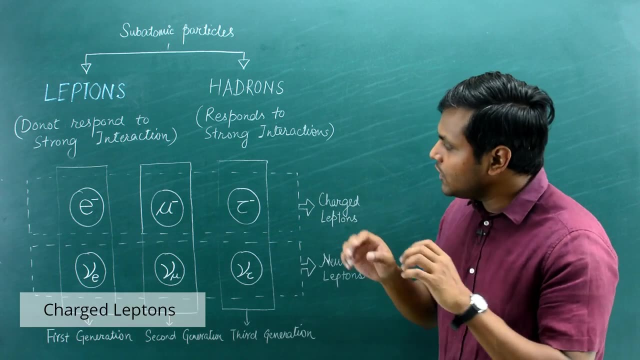 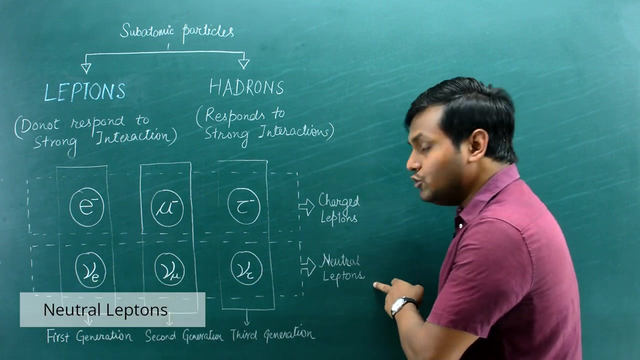 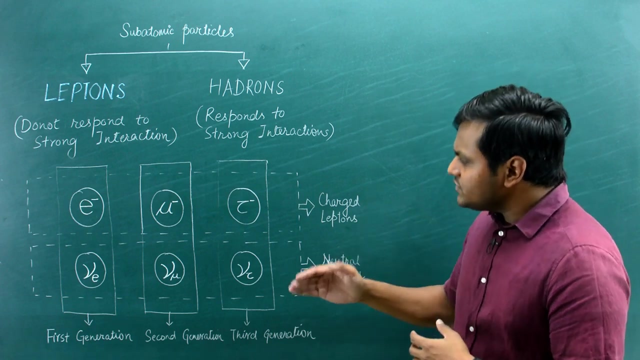 further organize them based on certain similarities. for example, the electron muon and the tau particles are known as charged leptons because they carry a negative electronic charge, while on the other hand, the neutrinos are known as neutral particles because they do not carry any kind of a charge. they are neutral particles, they have zero charge. so because of this reason. 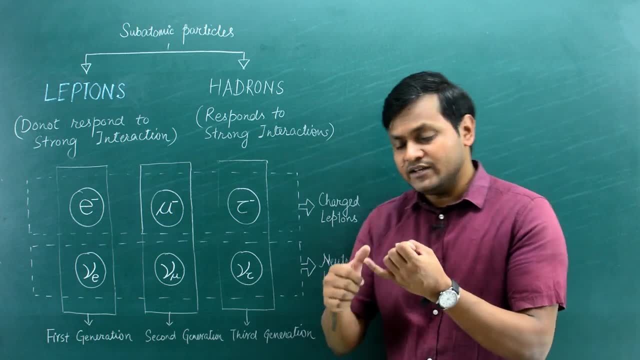 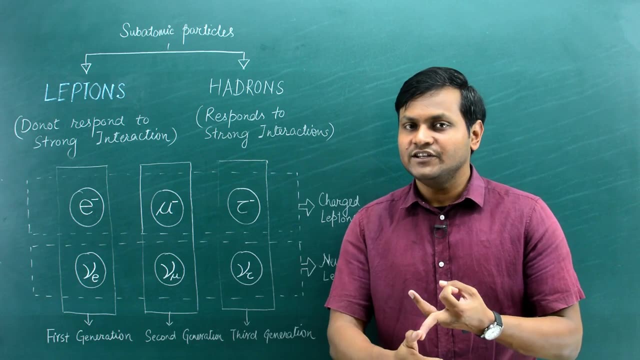 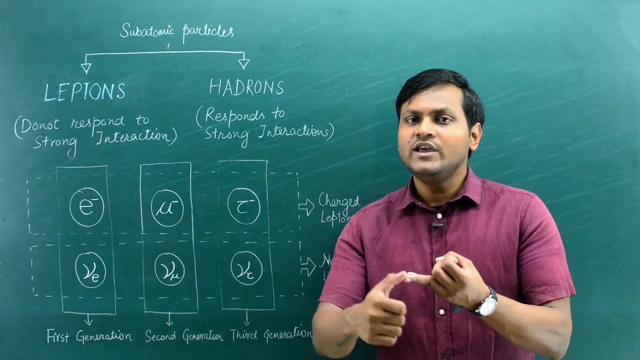 the charged leptons: they participate in gravity, they participate in weak interactions and because of their charge they participate in the electromagnetic force also. but on the other hand, the neutrino particles: they participate in gravity and weak interaction, but they do not participate in any kind of electromagnetic interaction. so in a sense these three particles, 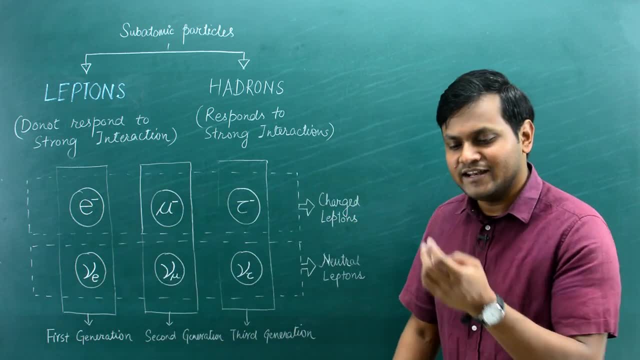 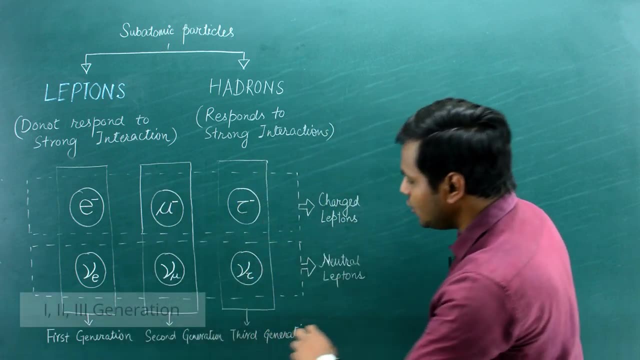 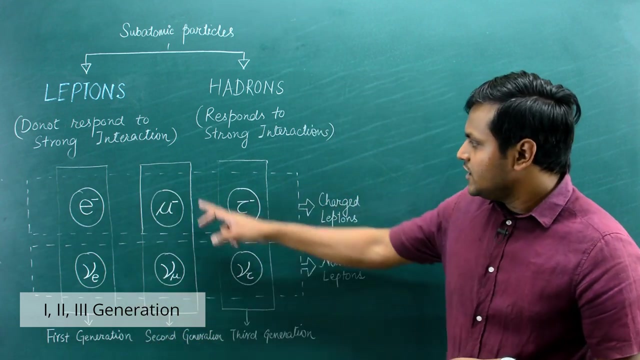 they only interact with three forces, while the other three particles they interact with two forces. furthermore, we can organize them into what is called the first, second and third generation of particles. so we have here the electronic leptons, known as the first generation, the muonic leptons. 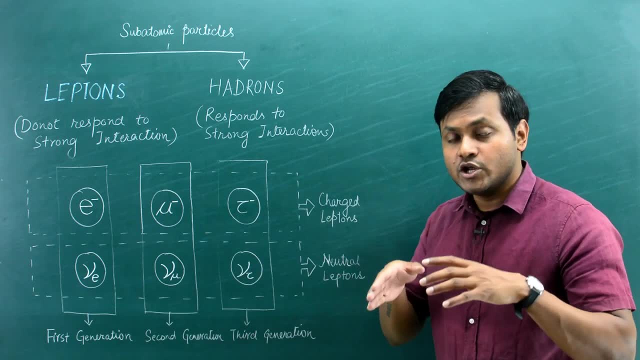 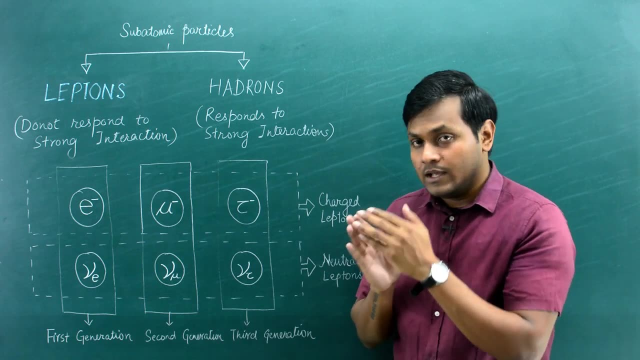 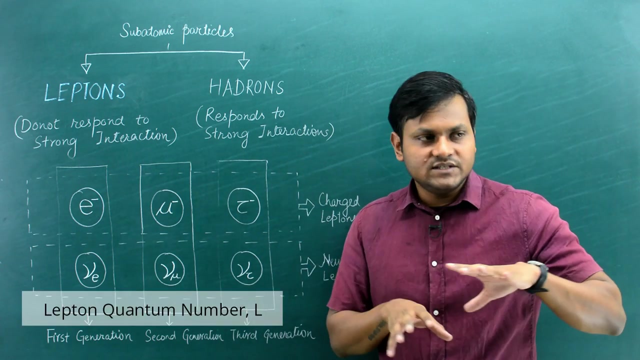 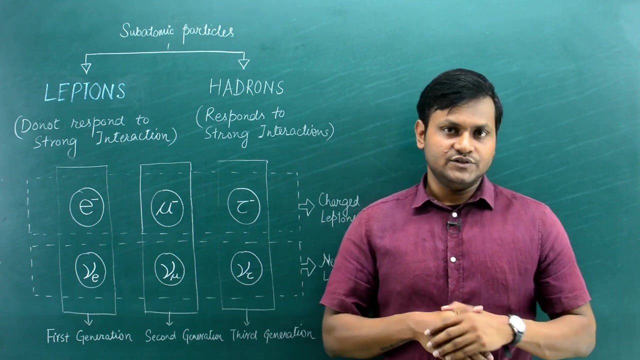 and the taonic leptons, known as the second and the third generation respectively. so each generation of particles are distinct from one another based on mass and also based on the lepton quantum number. so these particles, when they participate in different decay processes, there is a particular quantum number associated with the decay processes. so 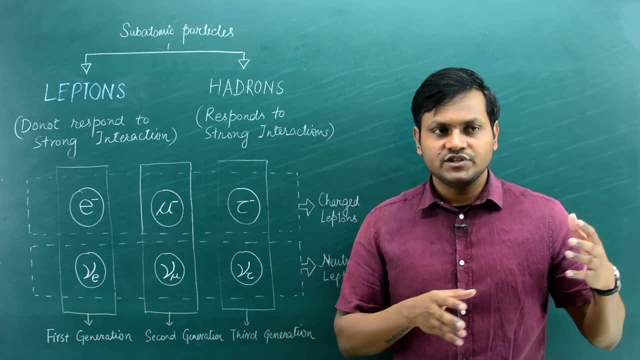 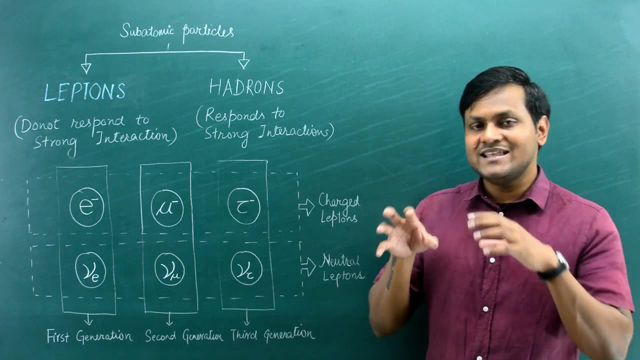 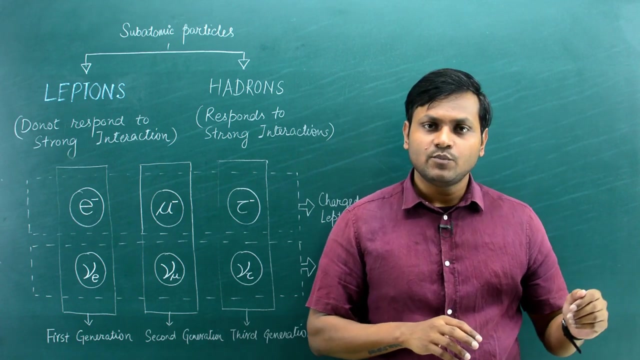 whenever some kind of elementary particle participates in decay processes, you have the usual conservation of energy, momentum, angular momentum, etc. etc. but for these elementary particles there are there are further quantum numbers that need to be conserved, which determine, mind, whether a particular decay reaction is possible or not. So lepton quantum number is: 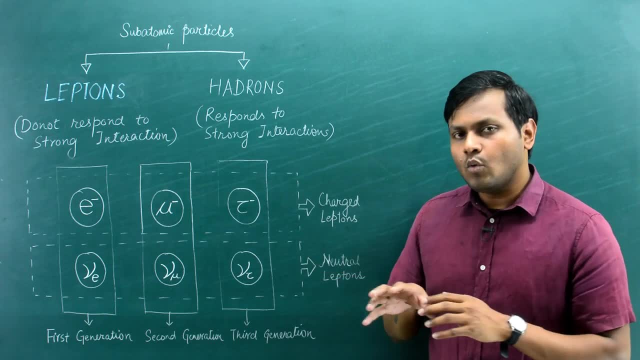 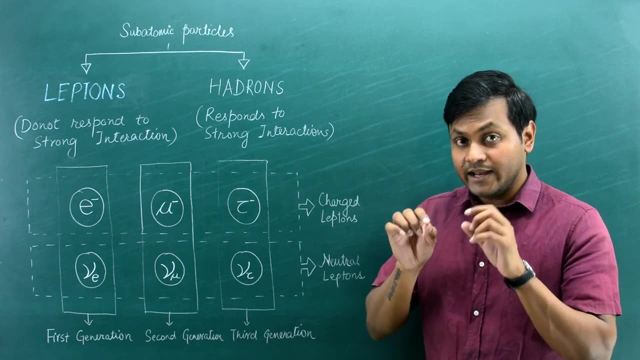 one such quantum number. I'm going to talk about this lepton quantum number in detail maybe in some other video, but for the time being, for this discussion, all I want to say is that there is a particular quantum number associated with the electron and the electron neutrino which is known. 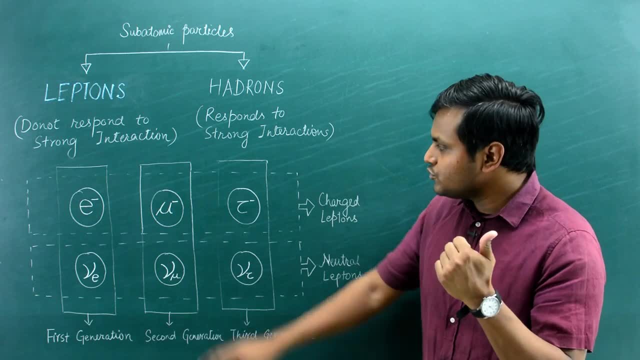 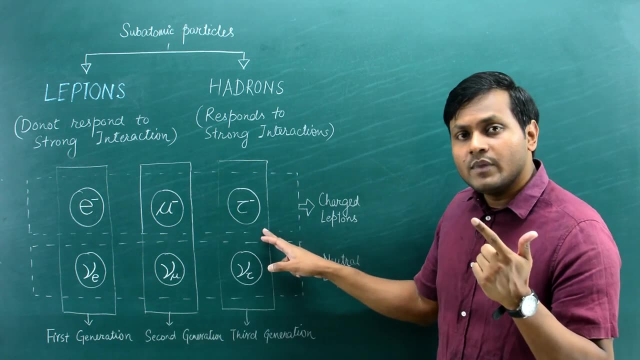 as electronic lepton number. There is another quantum number associated with the muon and the muon neutrino, which is known as a muonic lepton number, and there is another lepton quantum number associated with the tau particle and the tau neutrino, which is known as a tau lepton number. 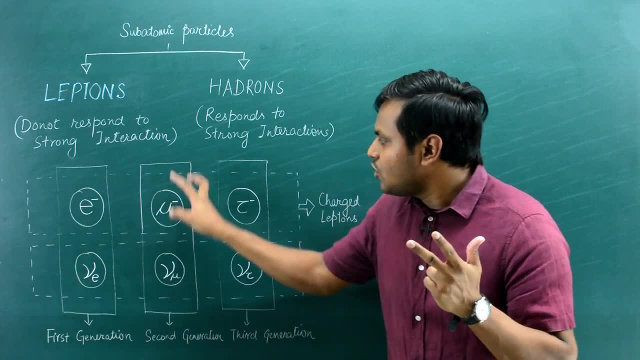 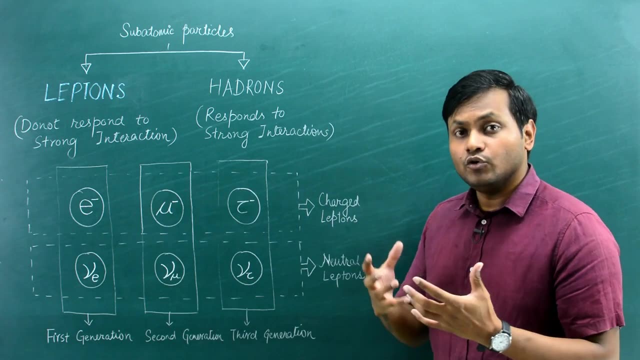 and these lepton numbers are associated with these, what is called first, second and third generation of leptons, by which we can further classify them. Also, the masses of each generation is greater than the previous one, so the third generation has more mass compared to the second. 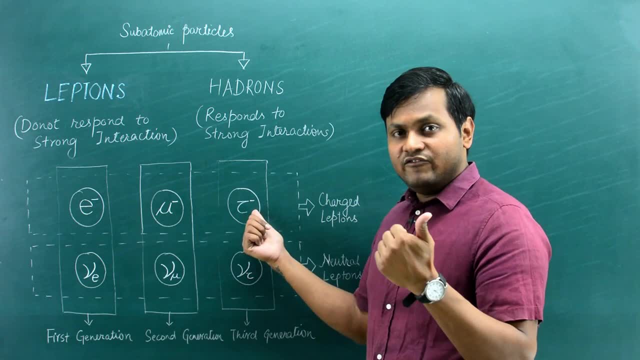 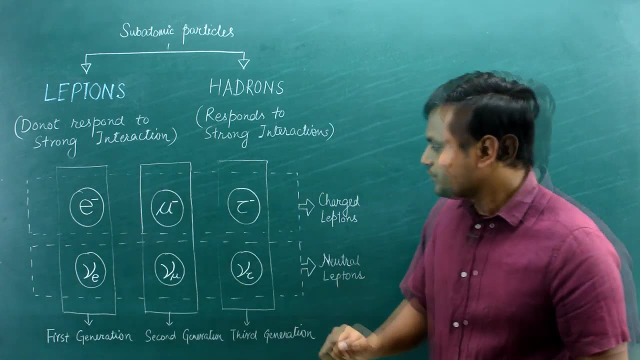 which has more mass compared to the first. So the tau particle is the heavier of them all, and the muon is lighter than the tau particle, and electron is the lightest of these three. On the other hand, as far as neutrinos are concerned, the masses of neutrinos, 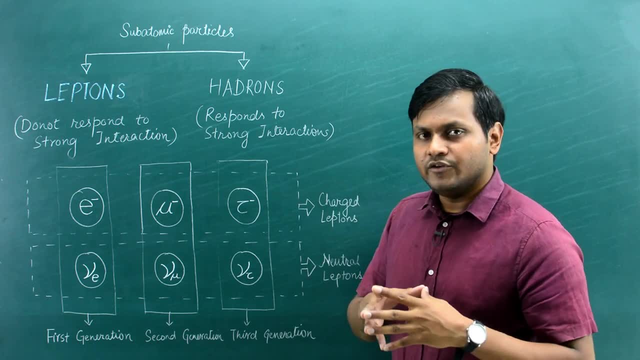 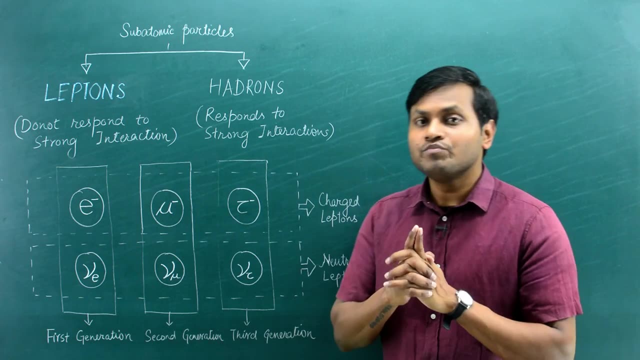 is still a topic of great interest in research in modern physics. so a final statement: as far as the mass of neutrinos is concerned is something that cannot be made Now. these neutrinos are attached, or rather associated with their individual charge, leptons like, so the tau. 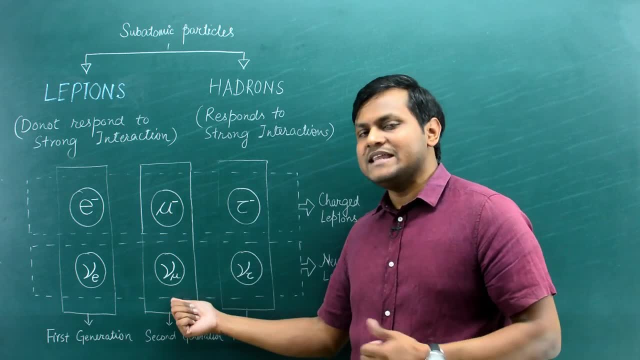 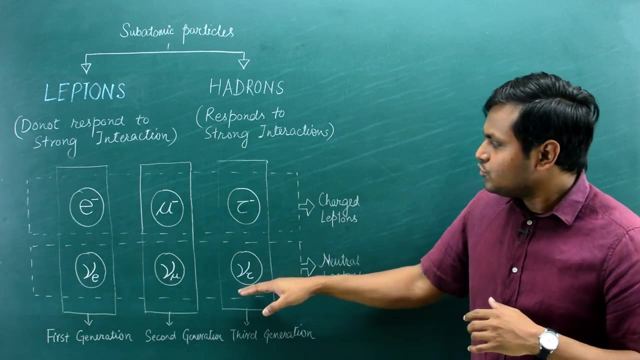 neutrino is named after the tau particle, which is known as the tau lepton number. So the tau particle, the muon neutrino, is named after the muon particle and the electron neutrino is named after the electron particle right. This is because they are associated with decay processes. 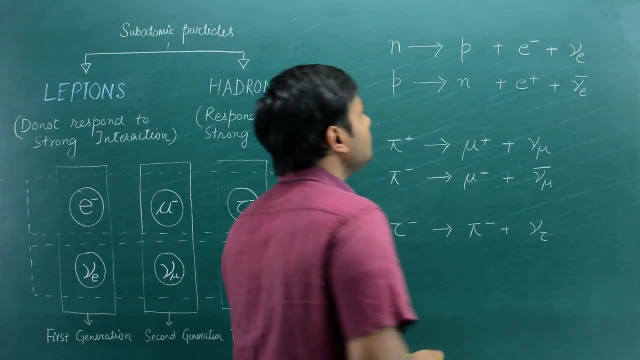 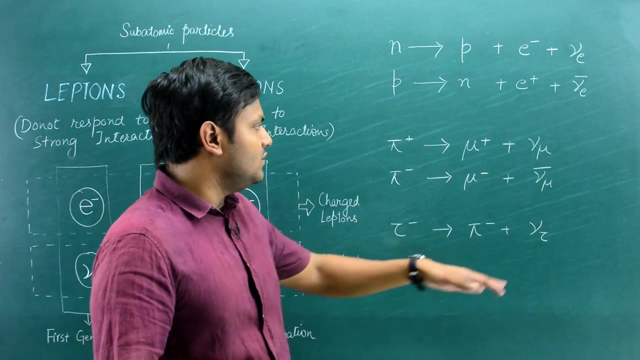 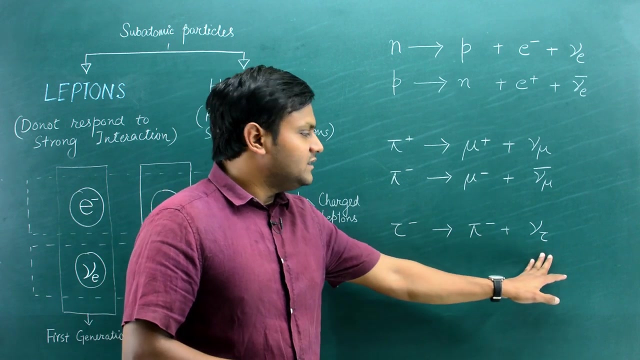 corresponding to these particles. So, for example, the electron neutrinos are associated with the decays of either electrons or their antiparticles, while the muon neutrinos are associated with the decays or interactions of either muons or their antiparticles, While the same for the tau 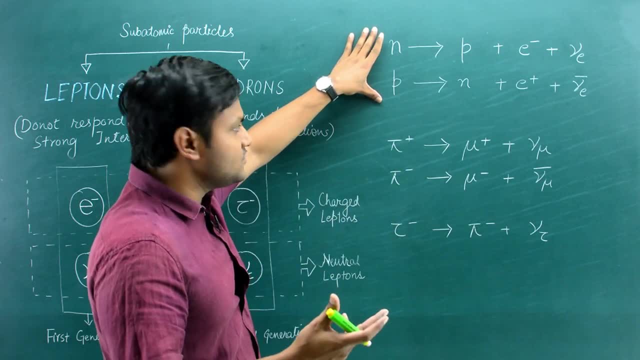 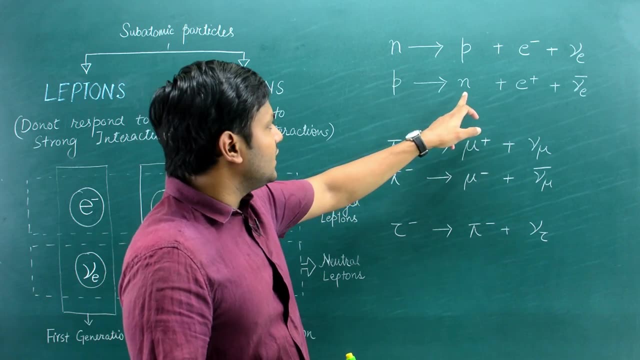 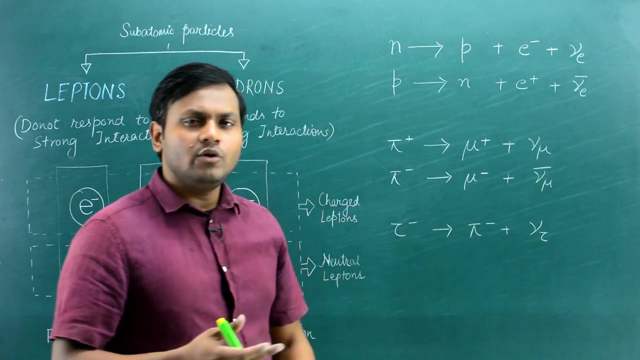 neutrinos, Like for example here, the normal beta decay processes that you have, where a neutron may get converted to a proton and lead to the emission of an electron, or a proton may get converted to a neutron and lead to the emission of a positron, are associated with the decays of either the electron neutrino. 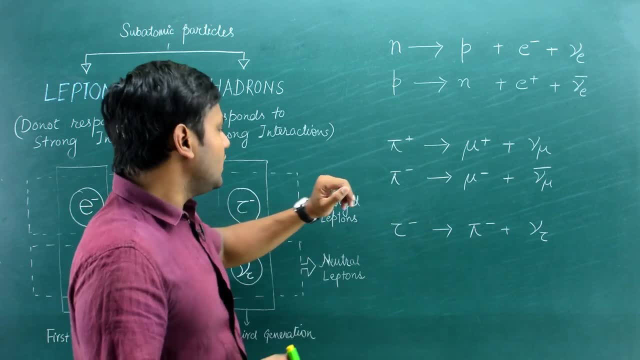 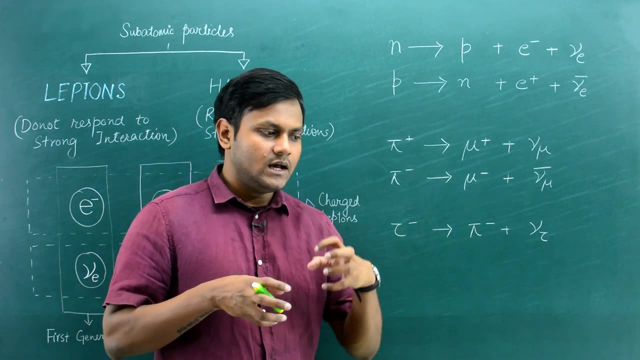 or its antiparticle, While on the other hand, for muon particles we may see a reaction something like a pi-mison getting converted to a muon. So pions are basically particles that are acting as a mediator between neutrons and protons inside a nucleus. 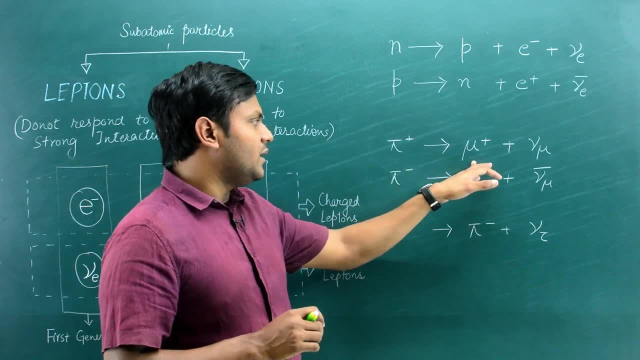 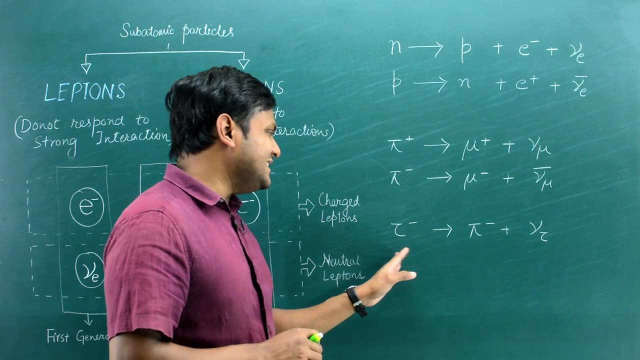 A free pion may decay into a muon particle and lead to the emission of a neutrino which is associated with a muon particle. Similarly, you can have a tau particle which may decay into a pi-mison and lead to the emission of a neutrino which is nothing but a tau neutrino. 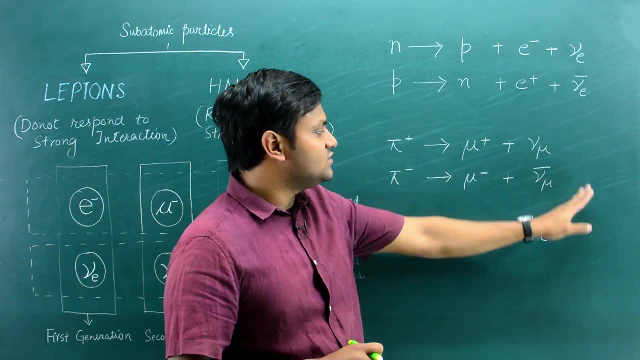 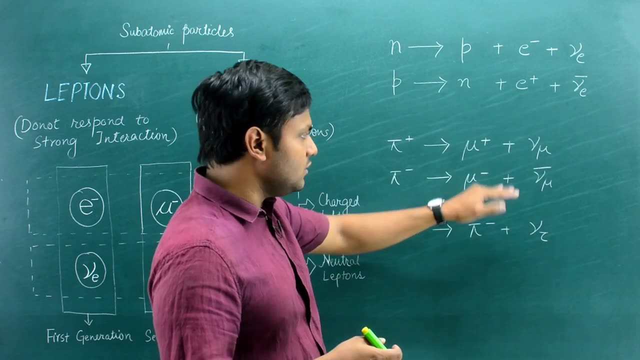 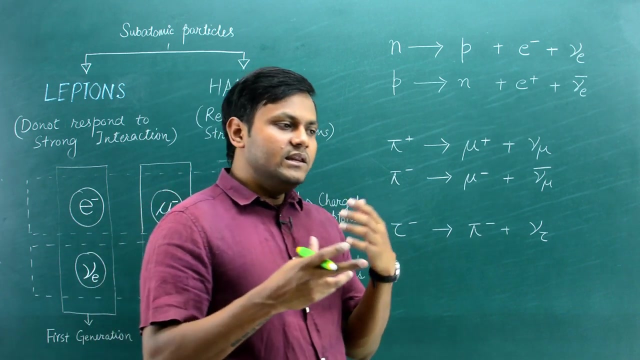 Now you may say that how are these neutrinos distinct from one another, or are they in fact distinct from one another? Yes, the neutrinos that are emitted alongside electrons or muons or tau particles Separately are quite distinct particles in the sense that they will lead to reactions. 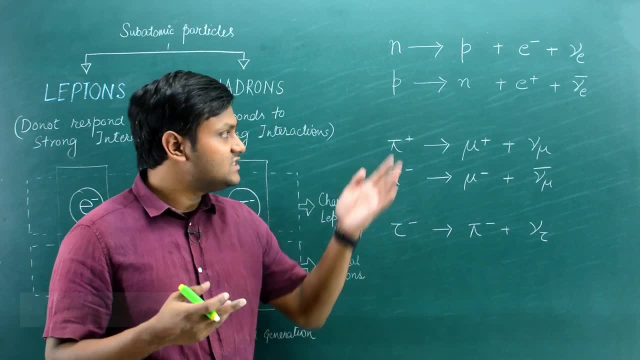 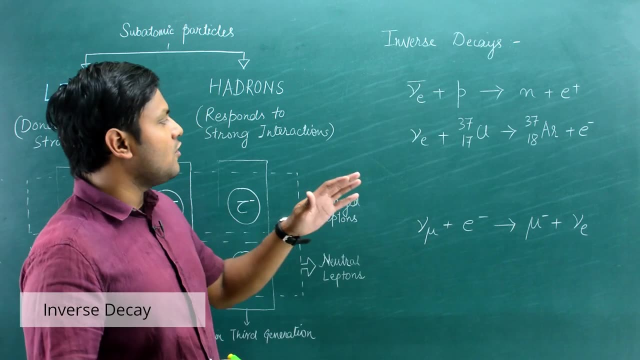 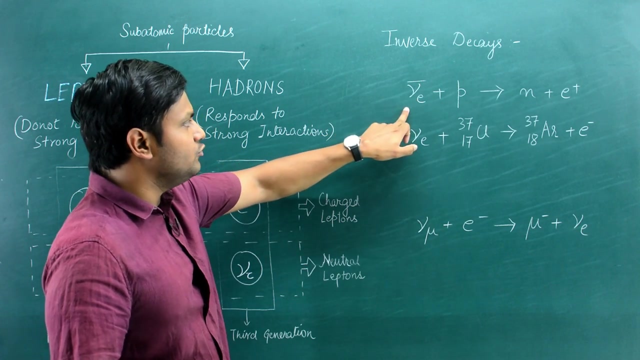 that cannot be interchanged. So, for example, if you look at the inverse decay processes corresponding to these antiparticles, The inverse beta decay, for example, consists of a neutrino interacting with either a- let's suppose- neutron or a proton. So in this case you have a anti-electron neutrino interacting with a proton that leads. 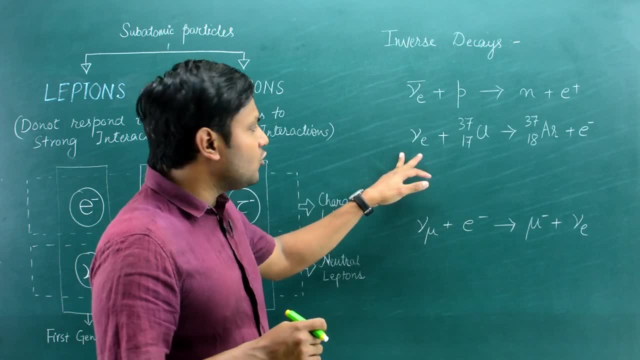 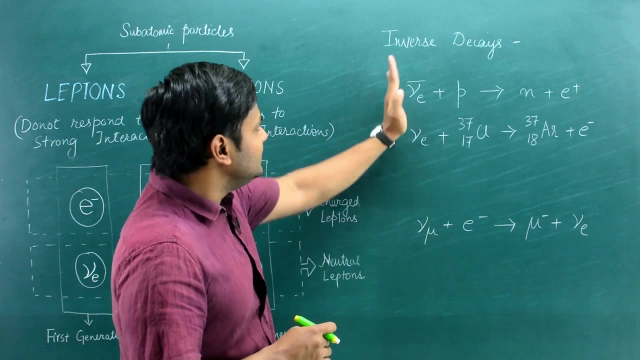 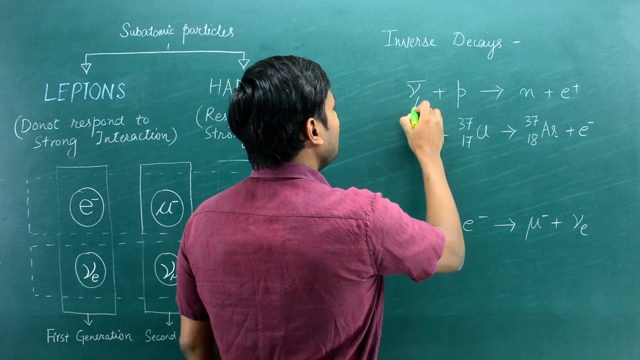 to the creation of a neutron and a positron. You can have another decay process Where a neutrino interacts with, let's suppose, a neutron in this nuclei to become a proton and an electron. Now these neutrinos are electron neutrinos. So, for example, if I replace this electron neutrino with a muon neutrino, then I will. 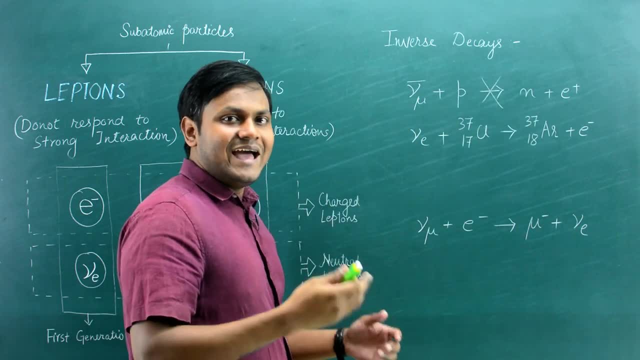 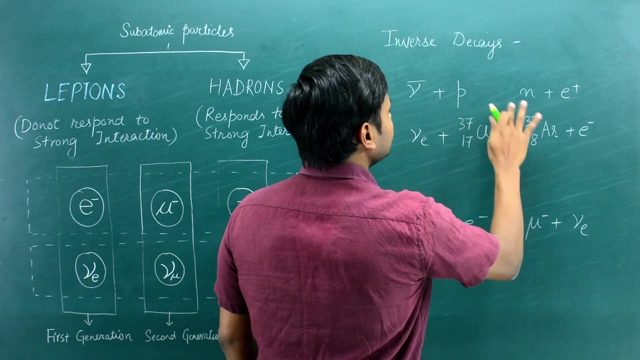 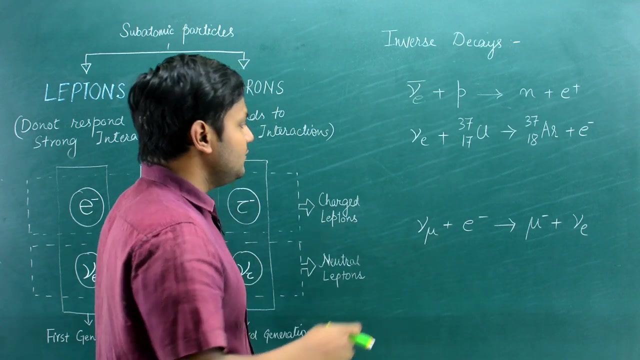 not get this kind of a decay process at all. Similarly, for this reaction, the only kind of a decay process, The only particle which can initiate this kind of a decay process of a proton converting to a neutron, is the electron anti-neutrino. So, for example, if you look at the decay process associated with the inverse muon decay. 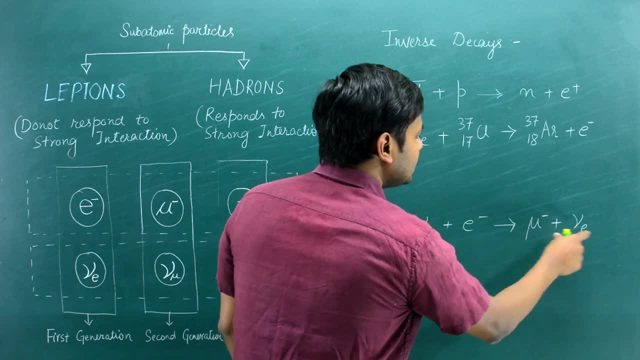 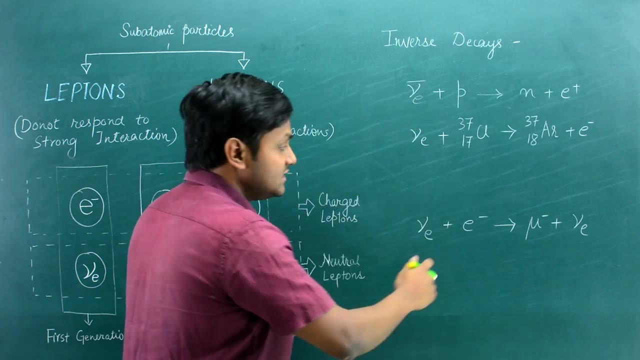 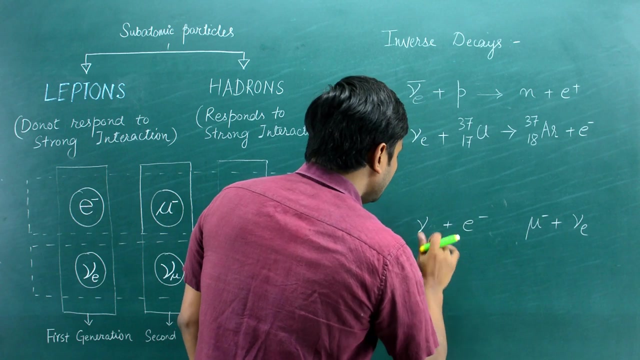 So a muon neutrino interacts with an electron to become a muon particle and an electron neutrino. in this case I cannot have a decay process with the electron neutrino. in this case This decay process is not possible. I can only have a decay process like this with a muon neutrino. 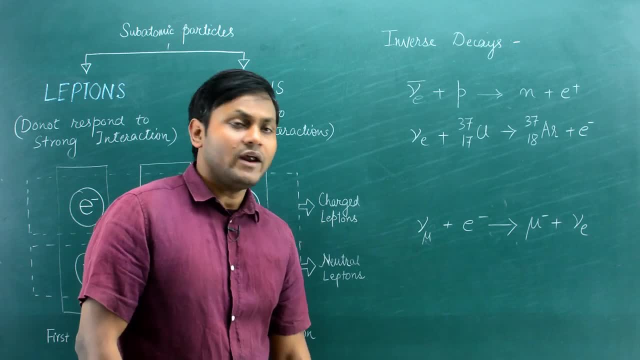 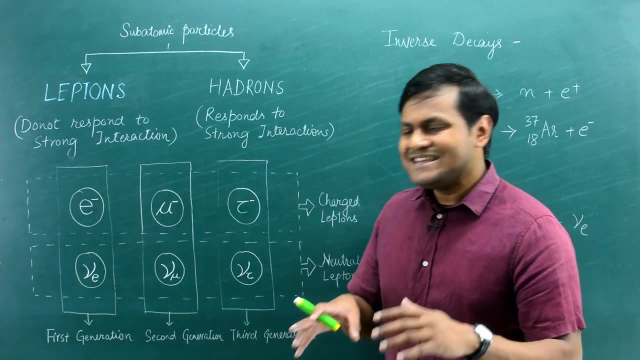 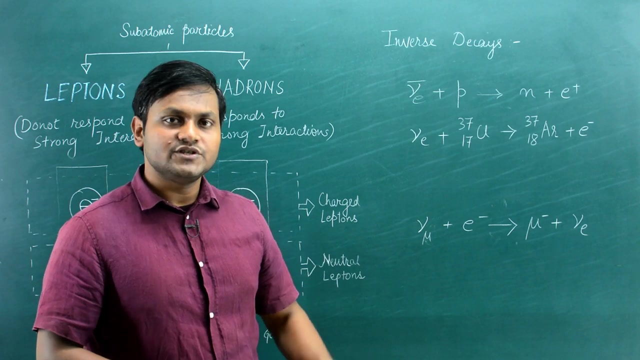 So this is a decay process, which is the inverse muon decay. So because of this reason, we can say that these electron, muon and tau neutrinos are quite distinct from one another. They lead to different kinds of inverse decay processes which are associated with the electron 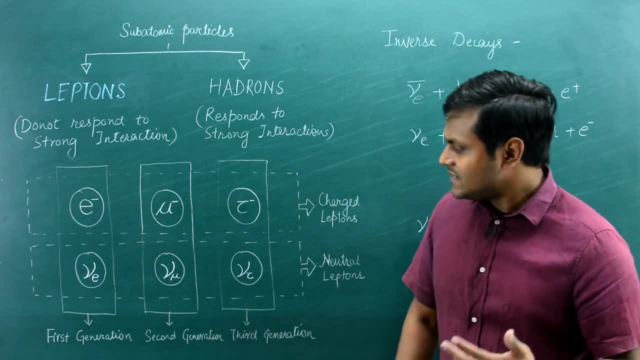 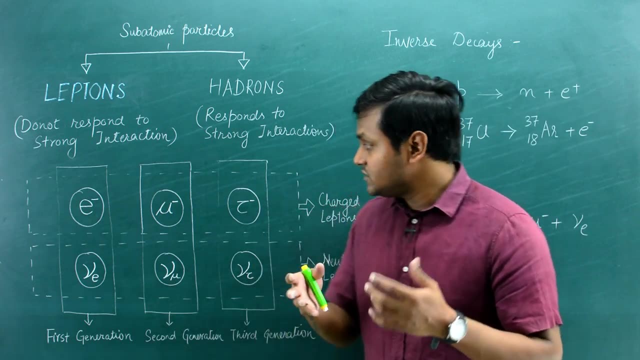 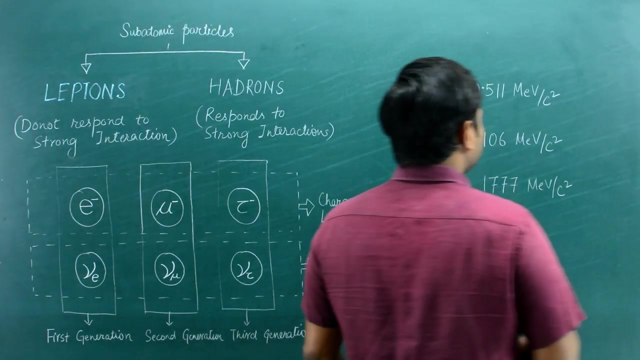 muon and the tau particles. Now I said that the first, second and the third generation of these lepton particles are distinct based on their masses, So one is heavier than the other, which is heavier than the first generation. So let's look at their masses. 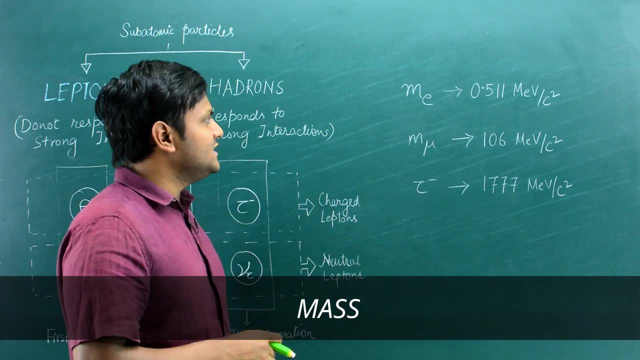 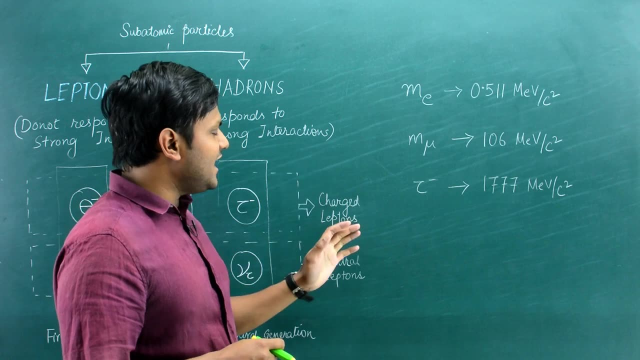 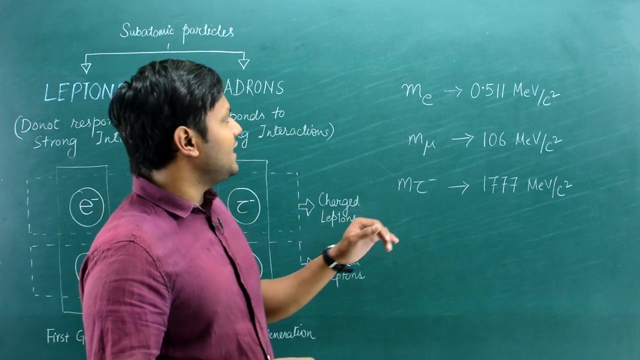 So the masses of these charged leptons are quite interesting in the sense that you have electrons, which is such a light particle. Its mass is very, very less. On the other hand, you have a tau particle, which is actually quite massive. So I have the numbers here for a comparison. 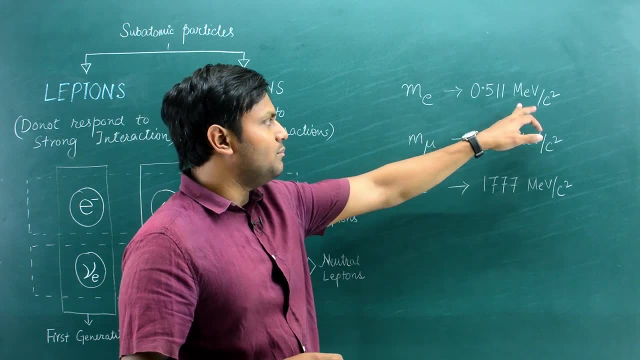 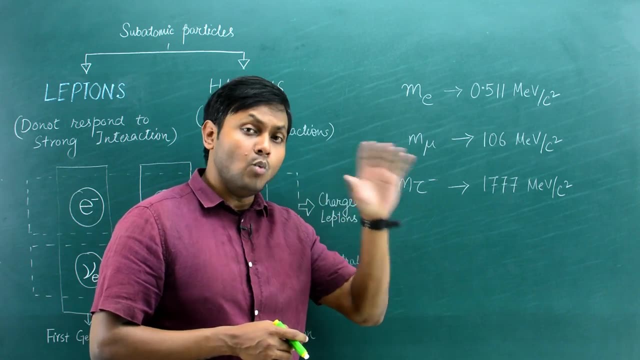 The electron has a mass of around 0.511 mega electron volt by 0.510 mega electron volt. So this is a mass of 0.511 mega electron volt. So in terms of kilograms it has a mass of around 9.1 by 10 to the power, minus 31 kilograms. 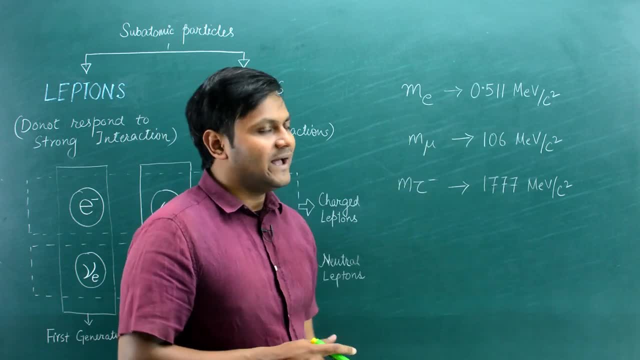 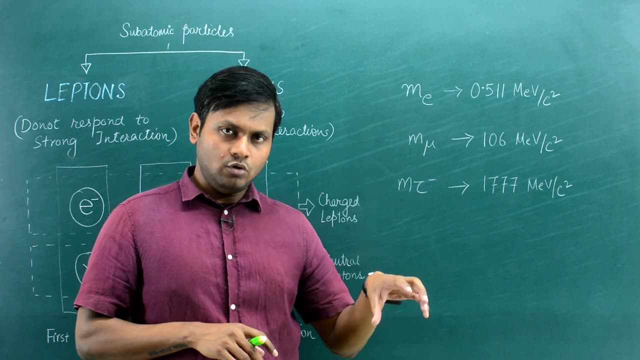 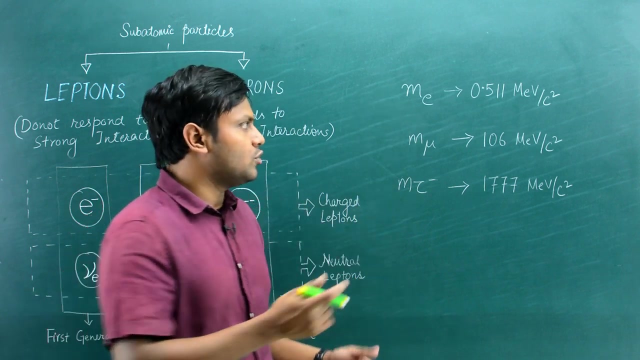 But in terms of electron volts we can write it as 0.511 mega electron volt upon c square. Now the mass of an electron. if you compare with, lets suppose, the mass of a proton, The mass of an electron is 1800 times lesser than the mass of a proton. 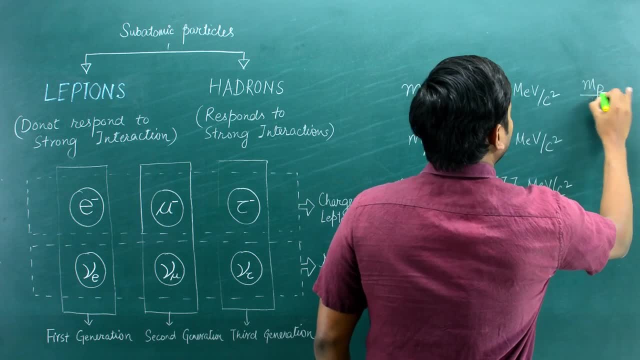 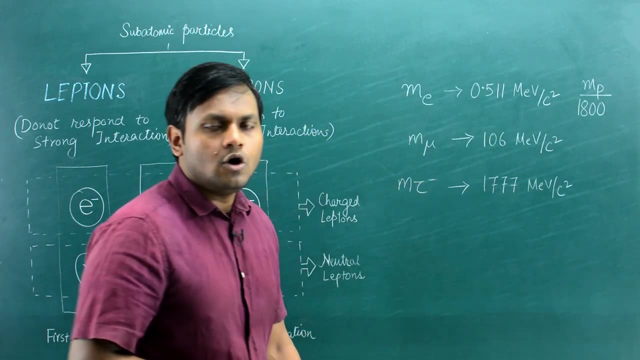 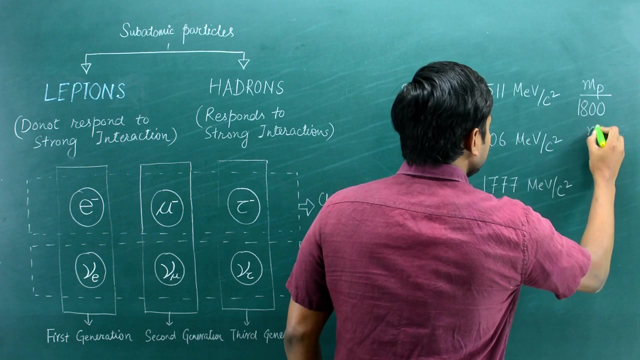 So, for example, the mass of a proton, The electron mass, is 1800 times lesser than the mass of a proton, 18, near, about 1800 times lesser than the mass of a proton. but if you do a similar comparison with, let's suppose, the muon particle, the muon particle is around 10 times lighter than the mass of a. 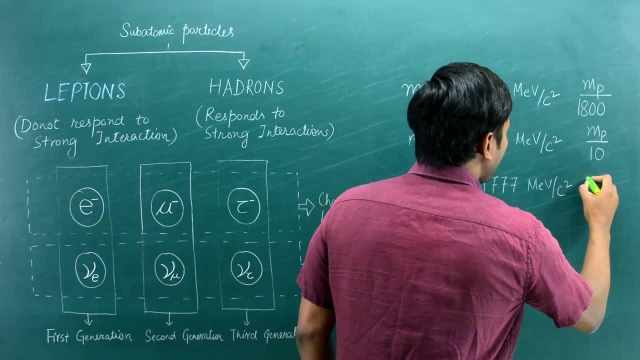 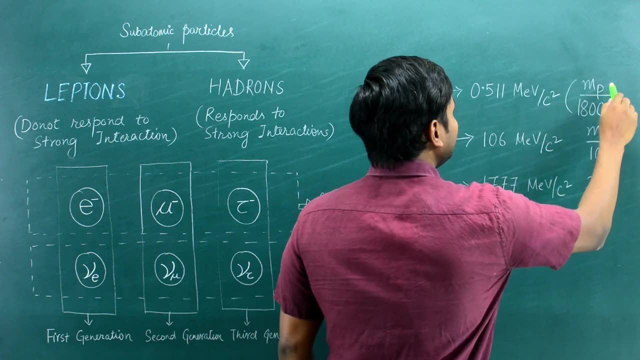 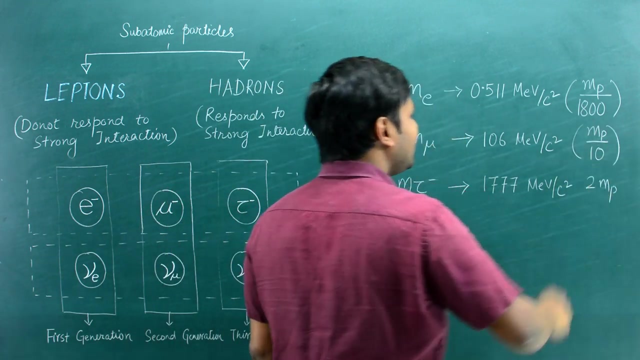 proton, while the tau particle is more massive compared to the proton itself, it's almost twice the mass of the proton, so the electron is almost 1800 or 2000 times lighter than the proton. the muon particle is 10 times lighter than the proton, but the tau particle is in fact two times more. 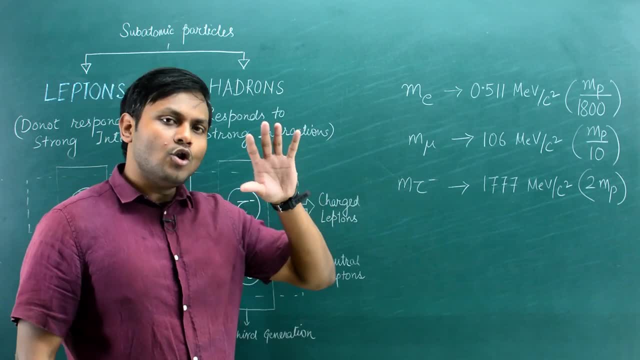 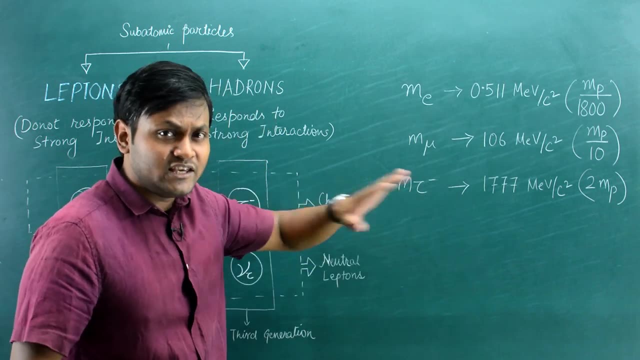 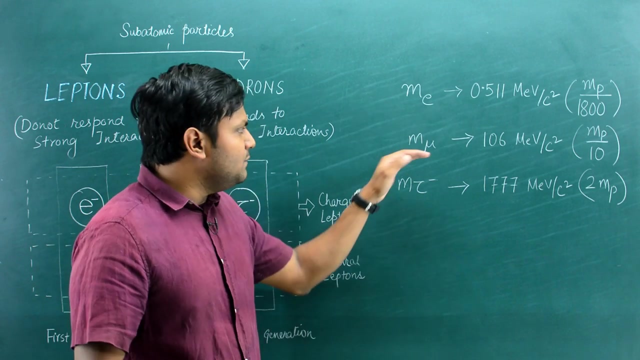 massive than the proton. so you see, the leptons are not always light particles. they have a huge range of masses. the tau particles are huge in the sense that they're very massive, in fact two times more massive compared to the proton mass. the muons are somewhere intermediate, 10 times lighter than 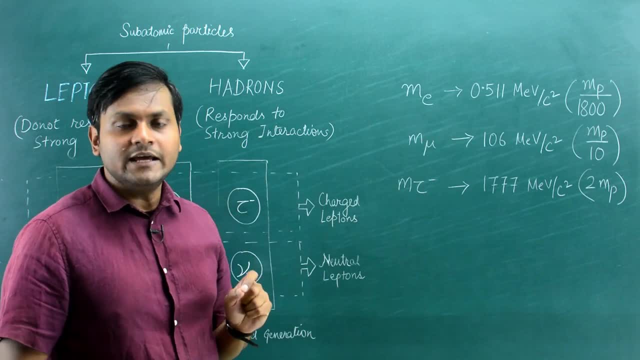 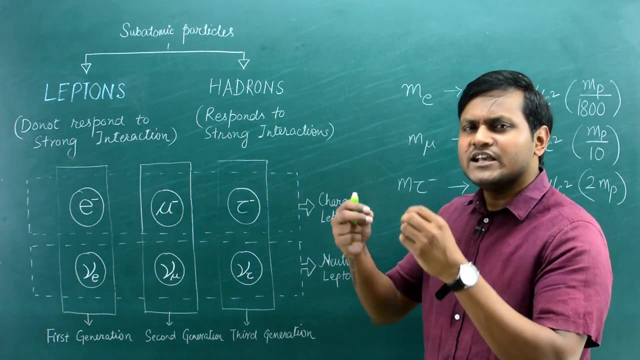 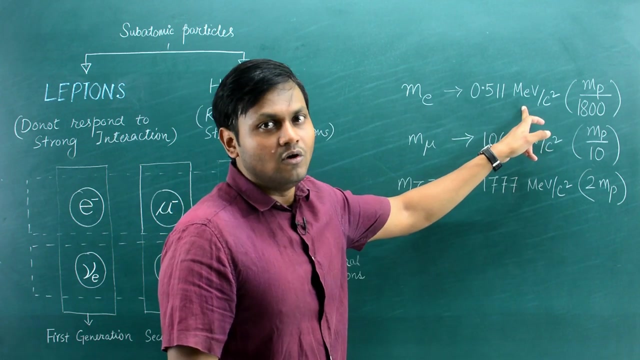 the proton mass, while the electrons are extremely, extremely light- they are 2000 times lighter than the proton mass- and the neutrinos, they are extremely, extremely light. if we talk about the masses of electrons, muons and tau in terms of mega electron volt, then if we talk about the 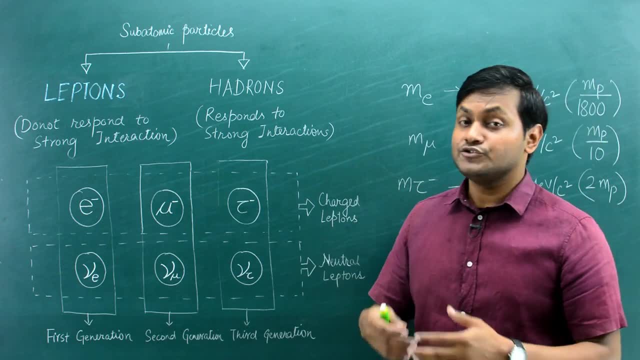 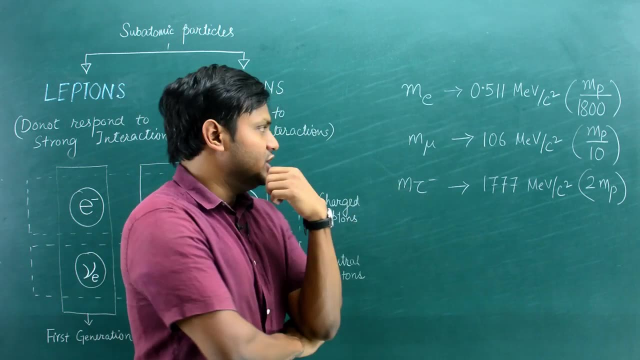 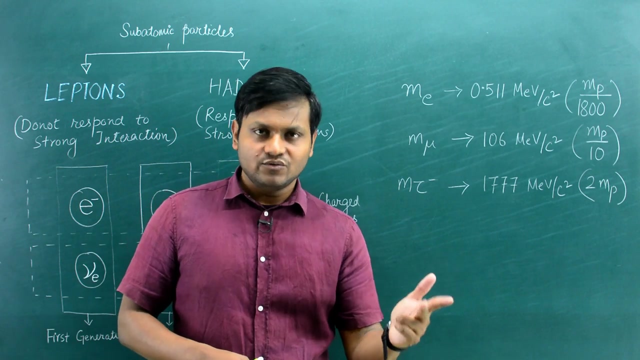 masses of neutrinos. they will be somewhere in kilo electron volts or even electron volt. now, usually we don't see the muon and the tau particles in nature. most of ordinary matter is made up of the electron. you see, the atoms are made up of neutrons, protons and electrons, mostly right. 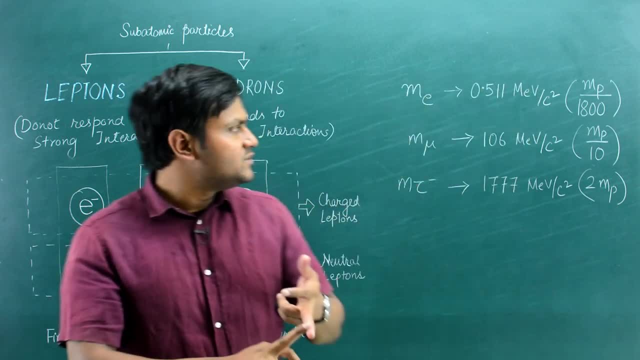 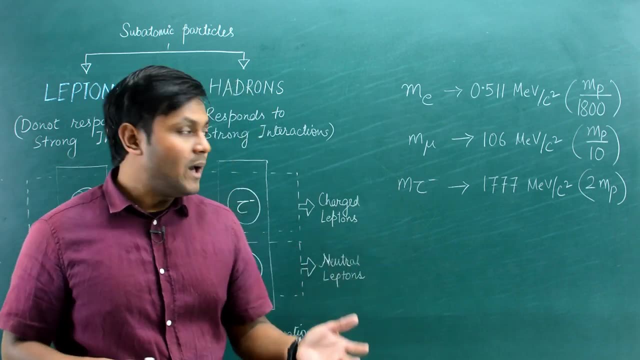 the neutrons and protons belong to the hedron family, the electrons belong to the lepton family. so electrons make up or electrons are constituents of ordinary matter. muons and taons are not. but muons and taons can get created in high energymandins. 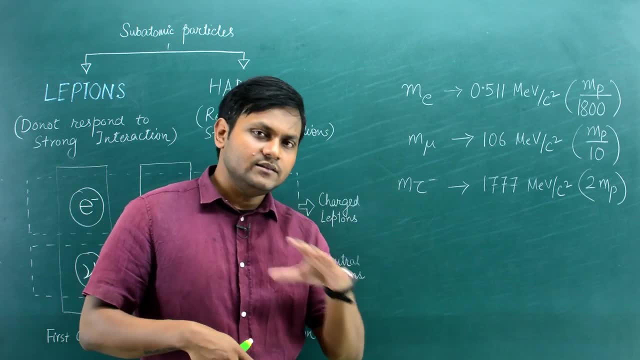 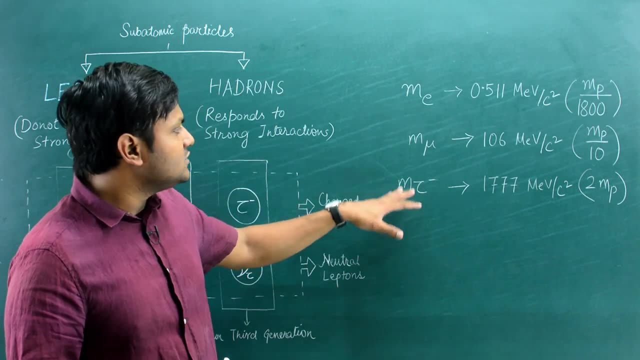 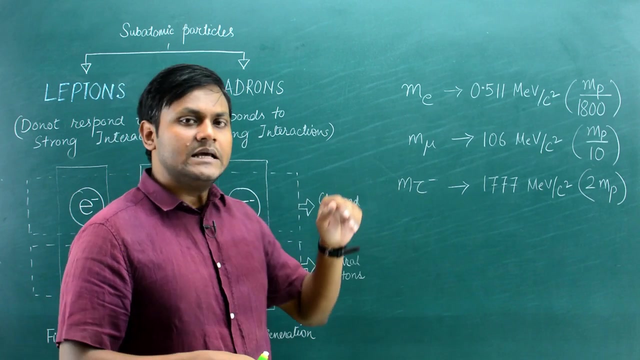 reactions like, for example, when cosmic rays hit the Earth's atmosphere or in particle accelerators where high energetic collisions are taking place. in those cases, muons and tau particles can be created. however, they are very unstable, so the muon has a lifetime of a few microseconds. where the tau particles 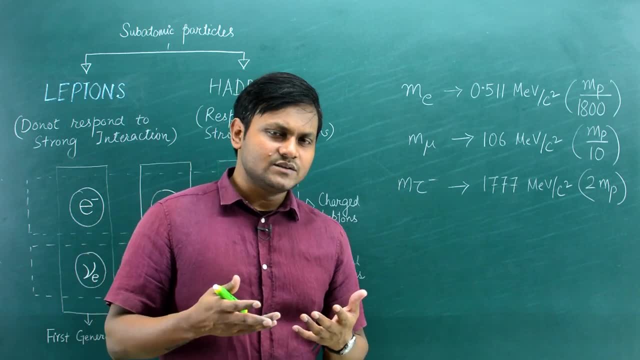 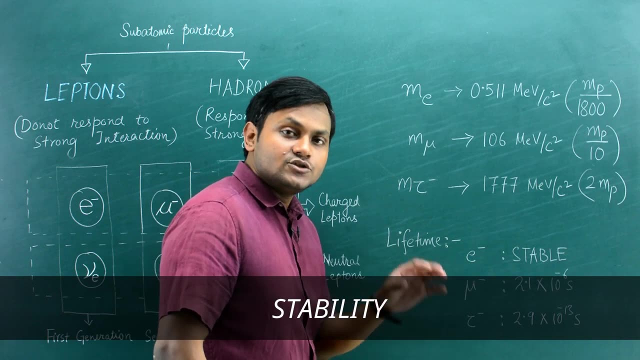 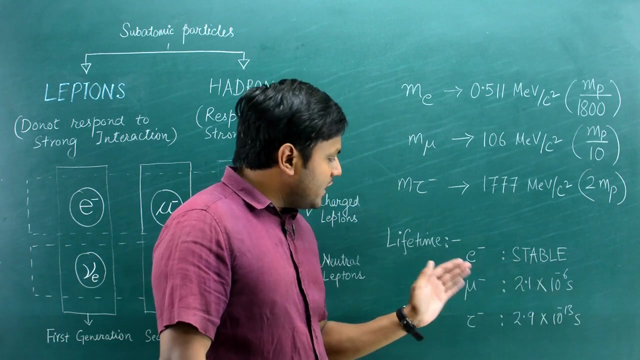 have a lifetime of even smaller time periods. so the tau particles have a lifetime of around 2.9 into 10 to the minus 13 seconds, so they decay in an extremely tiny time period, while the muon particles have a lifetime of around 2.1 into 10 to the minus 6 seconds. so whenever tau and muon particles are formed, either in the reactions involving cosmic rays or in particle accelerators, they immediately decay into a combination of other particles like neutrinos or maybe even electrons. electrons, however, are stable, so once in a decay process an electron is decayed, then the electron is decayed, and then the electron is. 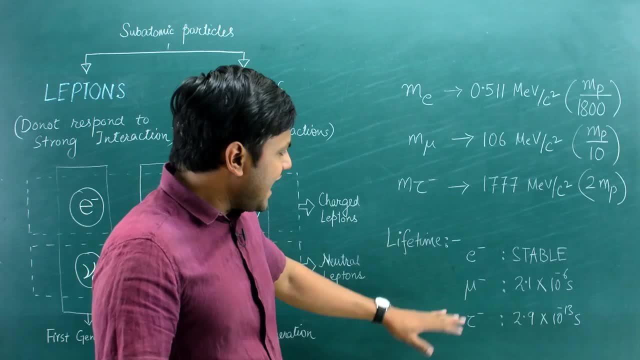 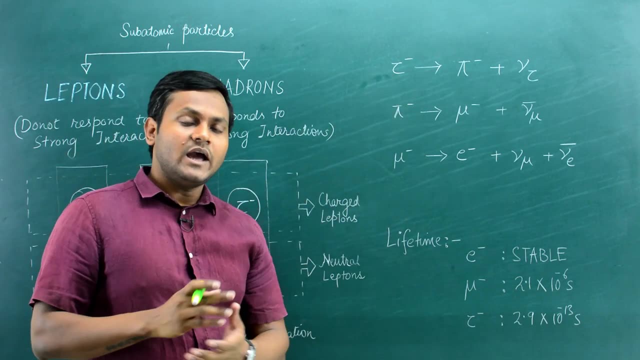 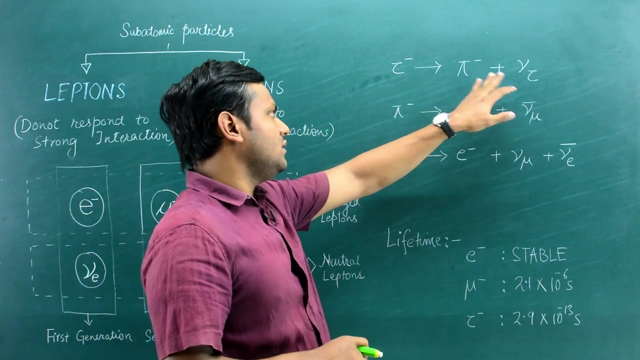 emitted. the electron is a stable particle, so we can look at some decay processes. so if a tau particle is, let's suppose, created in some kind of a high-energy particle accelerator reaction, then that would immediately decay into a pie meson and emit a tau neutrino. this pie meson may undergo further. 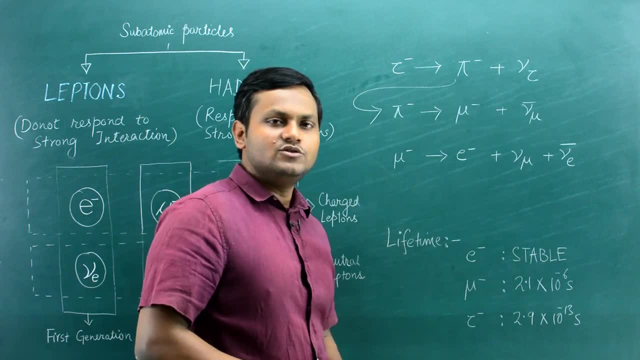 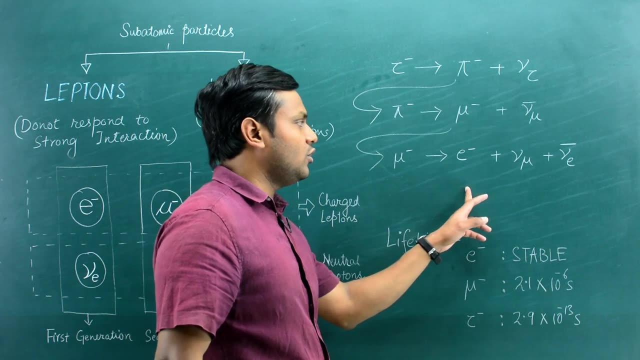 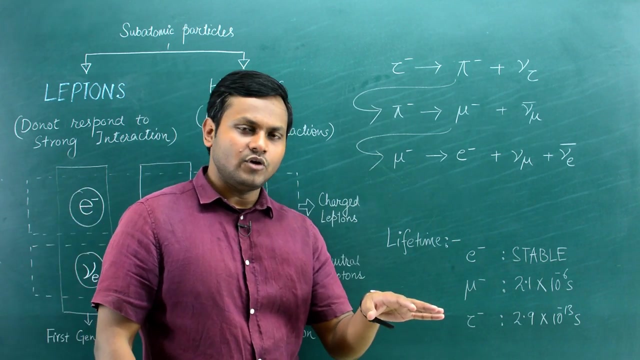 decay to a muon and lead to the emission of a muon anti neutrino. and the muon, which is also unstable, may further decay into an electron and two other neutrinos. so these are a few of the possible decay branches. out of many other possible decay branches, the tau might decay into a muon, which might 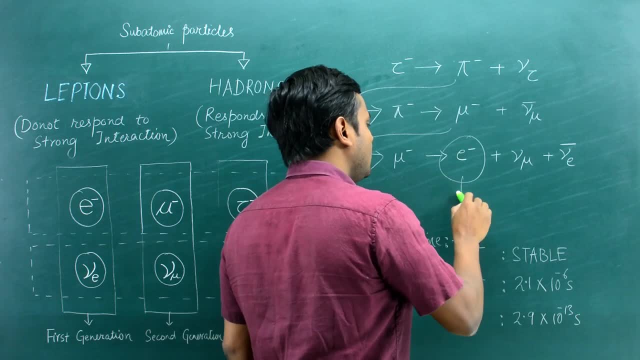 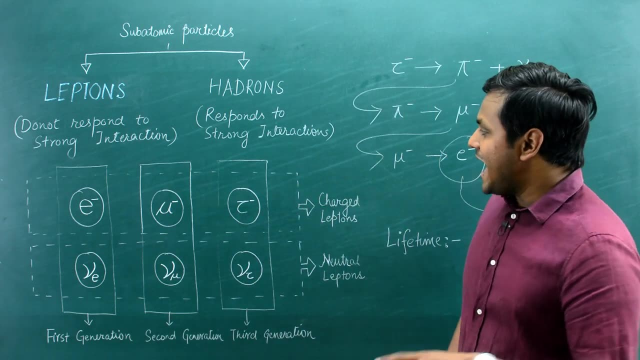 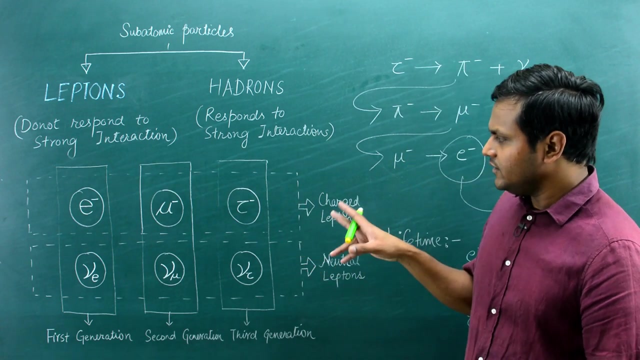 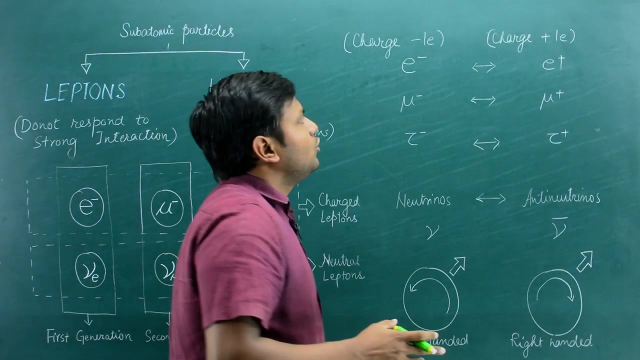 further decay into a very stable electron particle. so the electron is in fact one of the most stable as well as abundant charged leptons out there. now let's talk about another interesting property by looking at how these particles are distinct from their anti particles. so they charged leptons, the 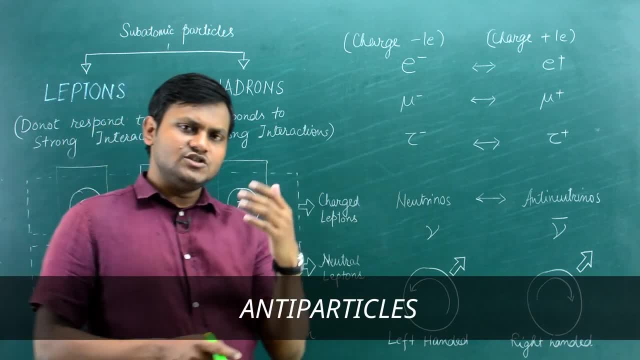 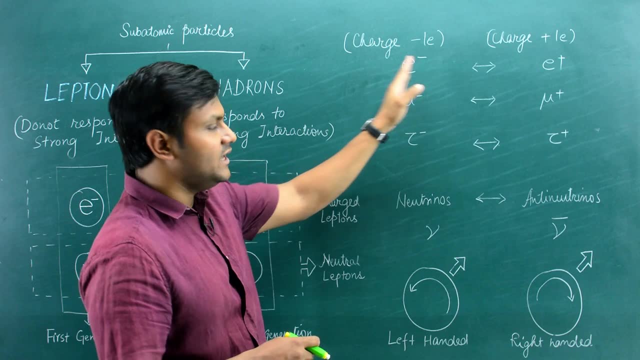 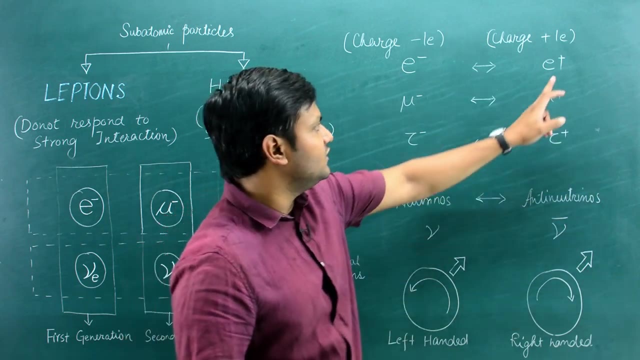 electron muon and our particle. they are distinct from their respective antiparticles based on the charge. so, as I said, the electrons, muons and time particles. they carry a charge of negative electronic charge. so the empty particles carry a positive electronic charge. that's why you have the plus sign here. on the case of electron muon and tau, you have the negative. 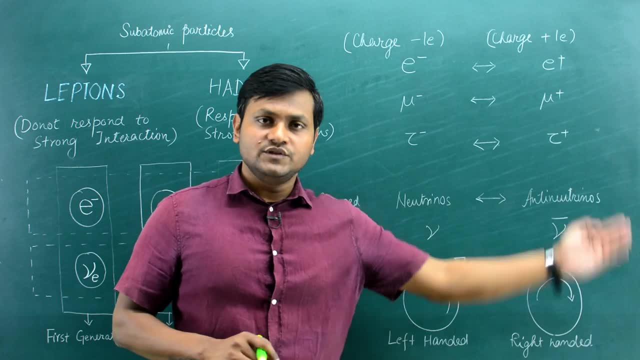 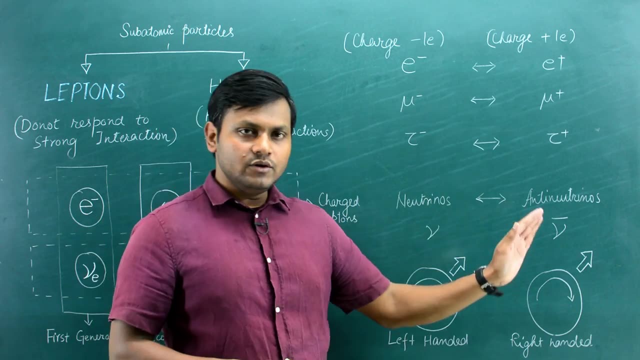 sign here. so they're distinct based on their charges. they have opposite charges. on the other hand, neutrinos, i said, are neutral leptons, right, they don't have charge. so how is it that neutrinos are distinct from anti-neutrinos? i've talked about this extensively in my previous video. 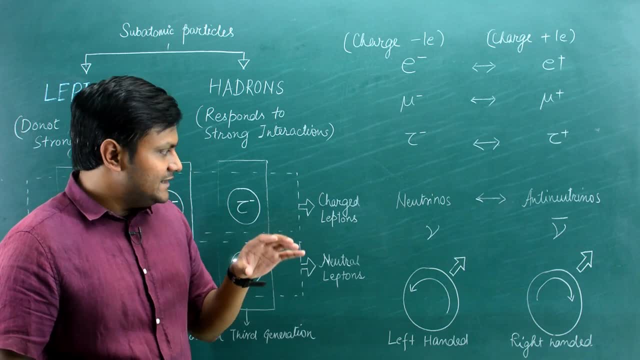 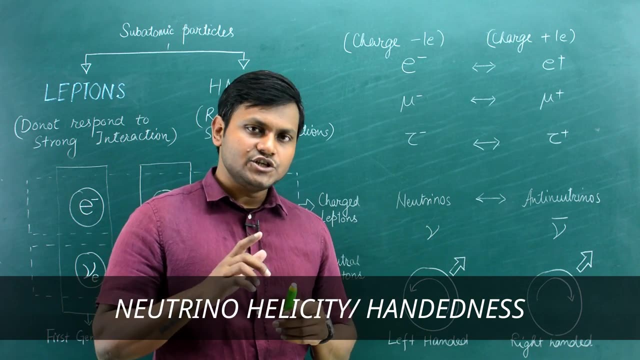 but for the sake of this discussion, let me just revise that neutrinos have a property called helicity. all right, so it basically gives us an idea about the orientation of its spin with respect to the direction of its motion. so neutrinos, it turns out, are left-handed, while anti-neutrinos 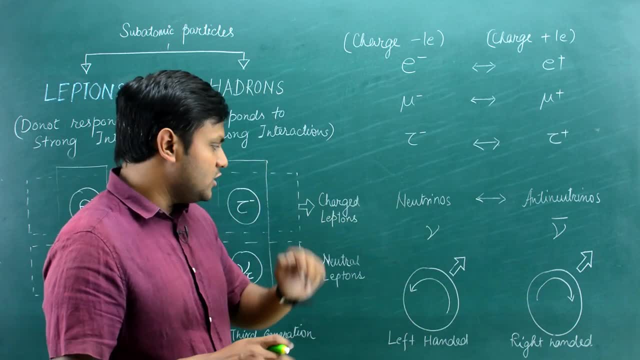 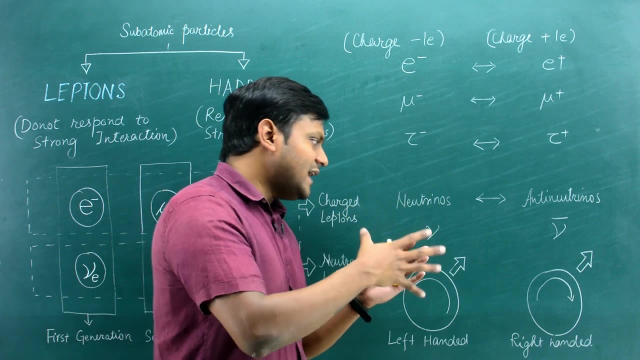 are right-handed so you can visualize this in this particular way. so if you imagine that a neutrino is penetrating this board or an anti-neutrino is penetrating this board, then if you're looking at these particles from behind, as these particles are penetrating the board- 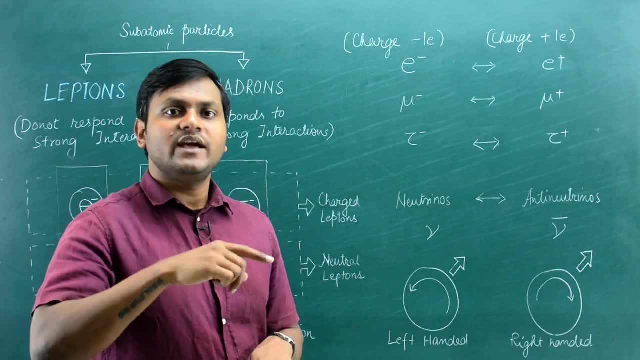 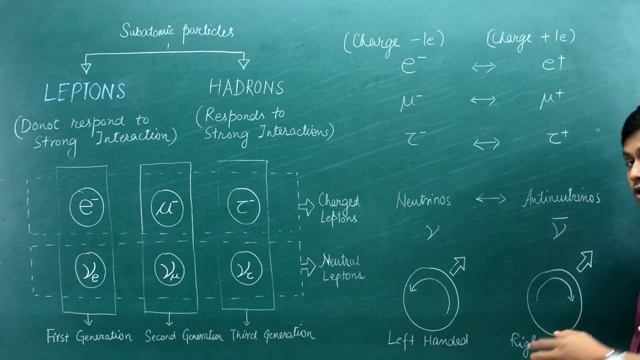 then you can look at the spin, whether the spin is in the clockwise rotation or an anti-clockwise rotation. so, for example, if you look at the anti-neutrino, you're looking at the anti-neutrino penetrating the board from behind. you can associate the orientation of 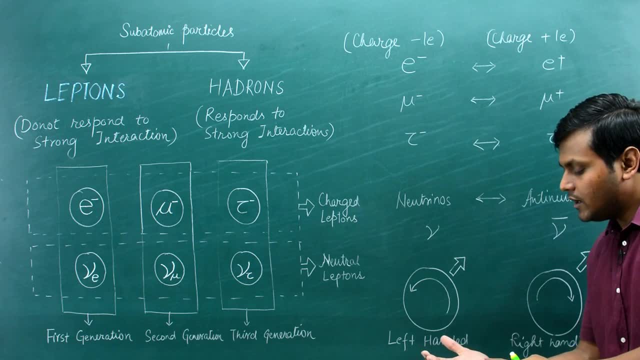 the direction of its motion with your thumb and the the curl of your hand with respect to its spin, by using your right hand. so if i take my right hand to represent the direction of its motion, which is the thumb going inside, and the curl which is the spinning, then this is called a right-handed. 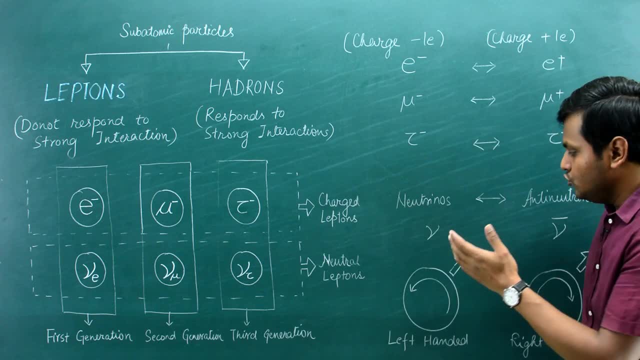 particle. on the other hand, if you look at the direction of its motion, then this is called a right-handed particle. on the other hand, for the neutrinos to represent the direction of your spin and the direction of motion, you'll have to use your left hand- okay, the thumb of your left and the 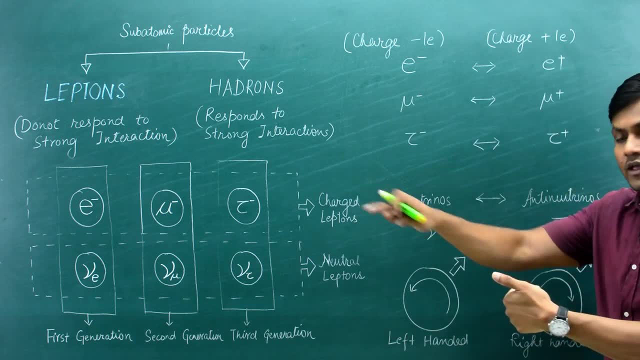 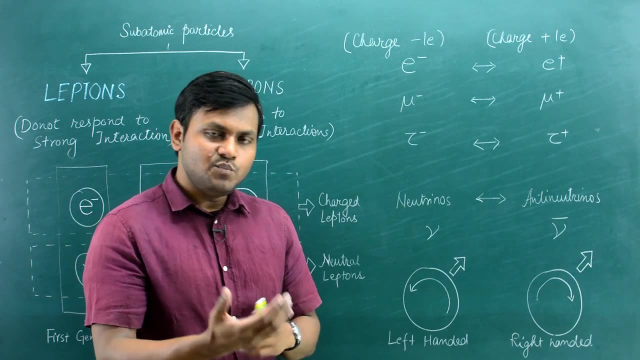 curl of your left hand represents the direction in which it is moving and in which it is spinning, as viewed from the back side. so if you can associate the spin and the direction of his motion with the right hand, it's called a right-handed particle, but if you can do it with the left hand, it's called a. 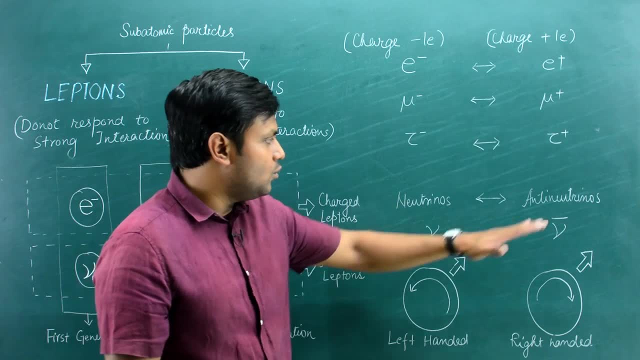 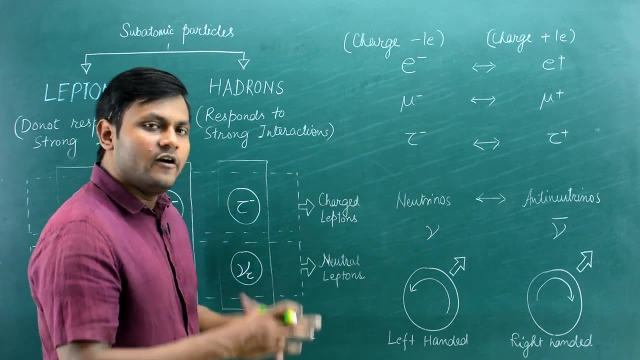 left-handed particle. so the neutrinos, as it turns out, are left-handed, while anti-neutrinos, as it turns out, are right-handed particles. so this is how the lepton family is distinct from their anti-particles. there is another property associated with these lepton particles, which is, as i said, 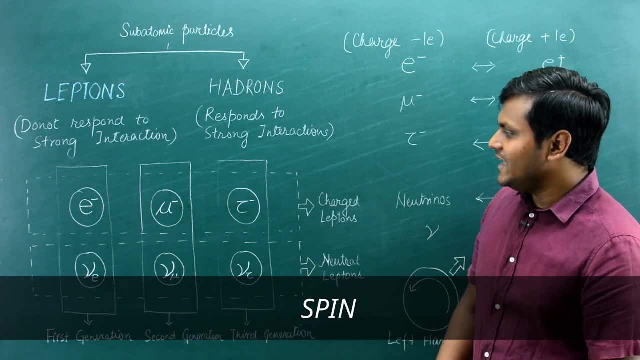 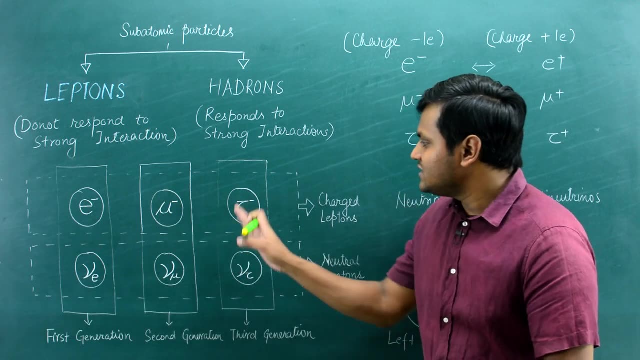 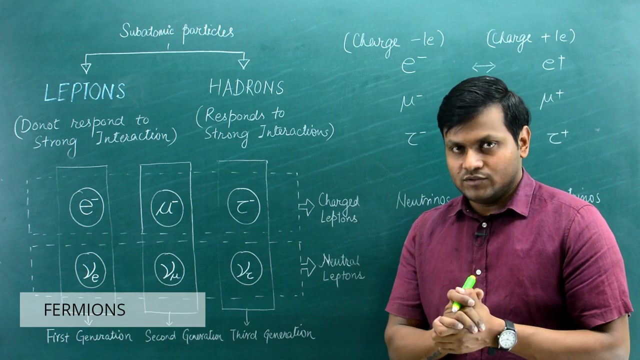 spin, right. so these elementary particles, they carry a particular spin, as it turns out, and they have a spin of half integer. that means electrons, muons, tauons, as well as the neutrinos have a half integer spin. so that means they are fermions, right, they are fermion particles. if you carry half integer spin, it turns out that you are fermion.